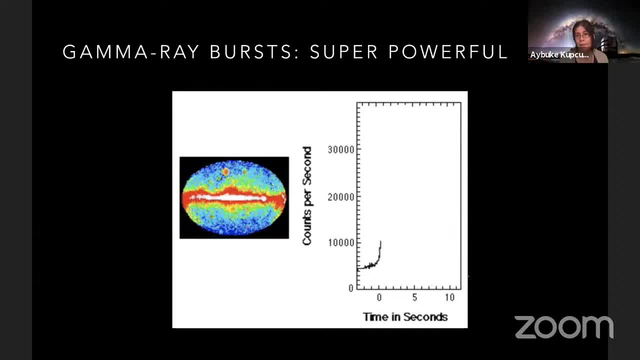 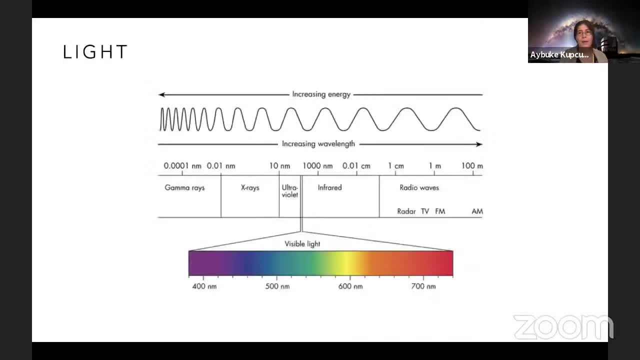 lighten up the entire gamma ray sky. So they are very, very powerful explosions. And gamma rays, just to give a recap, are basically very energetic light, high frequency, high energy light. And the light is basically a very large electromagnetic spectrum And we only see. 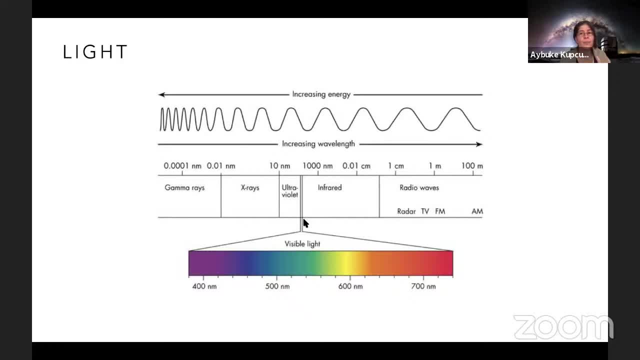 a little bit of it: the visible light, And on the one end, on the high energy end, lies the gamma rays, And on the lower energy range lies the radio waves, and like the FM and AM, for those who are old enough to remember, And so the gamma ray bursts happen in gamma rays, So there, 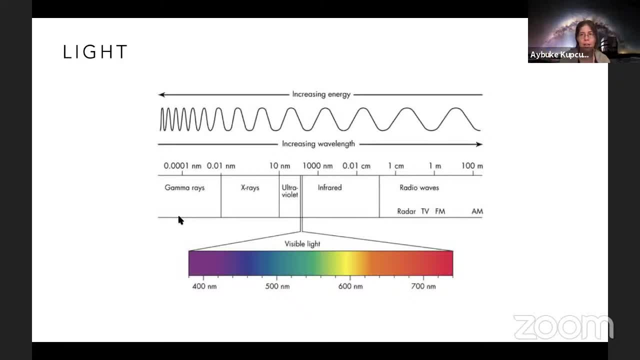 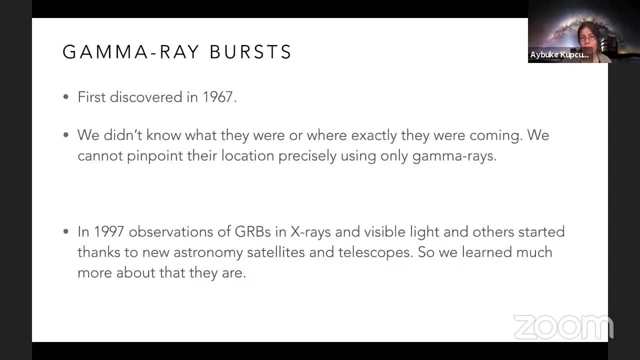 are these explosions that are happening in very high energy gamma rays lightening up the entire sky. They were first discovered in 1967. So they're relatively new. And and they were actually discovered during when the nuclear explosion surveillance. So while the satellites were surveilling the Earth to 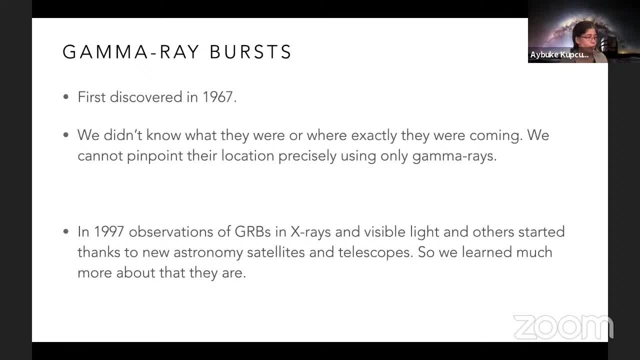 detect any. you know, nuclear explosion trials, and, but these were coming. these bursts were coming from the, from the space, But it's difficult to pinpoint the direction, the exact location of the gamma rays, And so therefore we actually didn't know, until 1997, what these were. So, and in 1997, the Compton satellite was started. 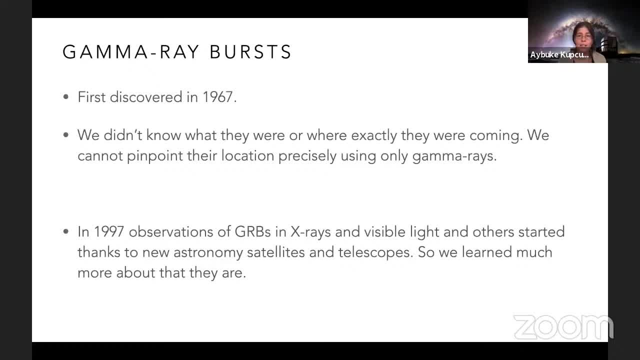 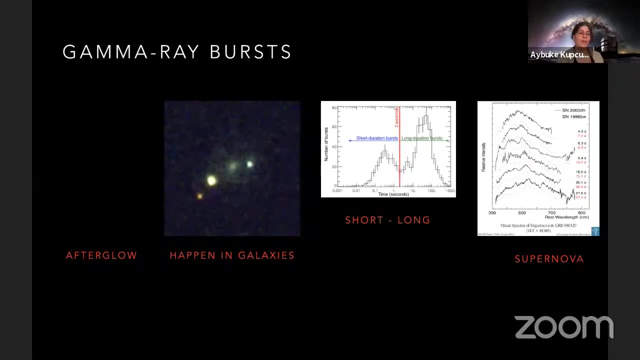 observing, And after the gamma rays, it detected x rays and visible light and other wavelengths, And so the gamma rays were coming from the same location, And that's how we started to learn much more about what the gamma ray bursts are. So I don't know why this one is not showing, Sorry. So there is. 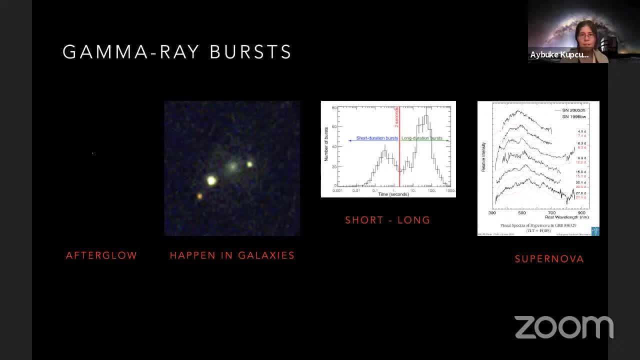 an afterglow emission from the gamma rays, As I said. basically there is some again sort of bursting light that decays within a few minutes to a few day, days In x rays. for some gamma ray bursts it's also visible in optical, so visible light, infrared and even radio. So and it also decays. they all decay in time and disappear eventually And this is why we called afterglow. they just happen right after the gamma ray burst itself And we also know they- oh sorry, oh, there it is. 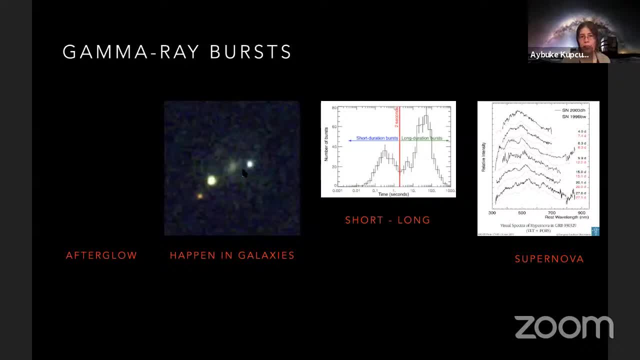 And they also happen in galaxies, So this should be the one. Yeah, Basically, as you can see, this one is actually the gamma ray burst in the optical and near infrared light, and it actually lies on one of the spiral arms of this galaxy, So it fades away The. this is the afterglow emission in the visible 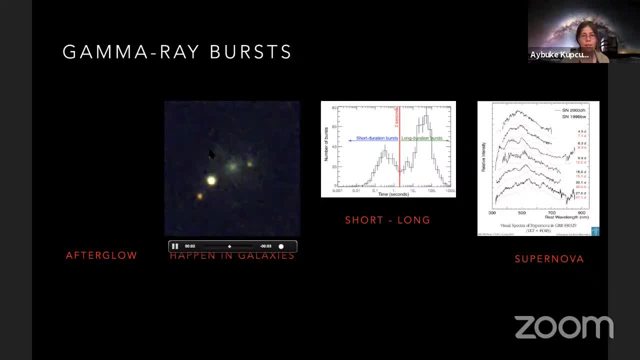 light and near infrared lights, And once it fades away, we can see the galaxy much better with this spiral arms. This is the one of the images taken with the Hubble telescope. We also know that they belong to kind of they're divided into two categories. 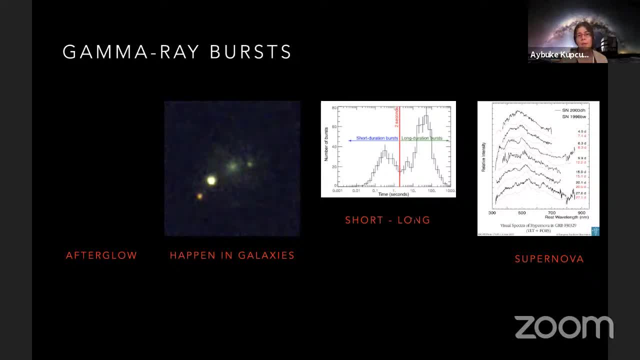 according to their duration: the duration of the actual gamma ray explosion, the burst. Roughly the ones that are shorter than two seconds are called short gamma ray bursts and longer than two seconds are called long gamma ray bursts. And this is not only because 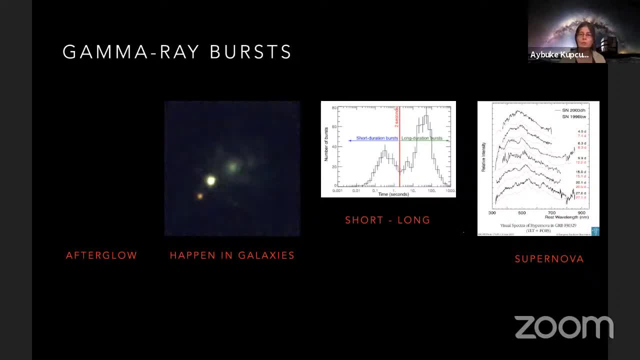 there is this distinct division in terms of duration, but also they have some other different properties. For instance, the short gamma ray bursts don't necessarily show that much of afterglow emission and the burst itself seems to be in harder gamma rays, And we also see supernova explosion at the same time. 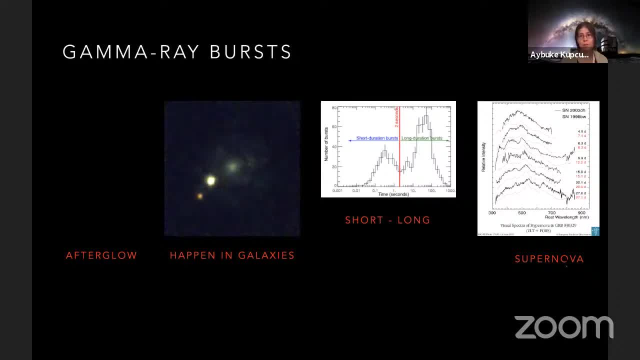 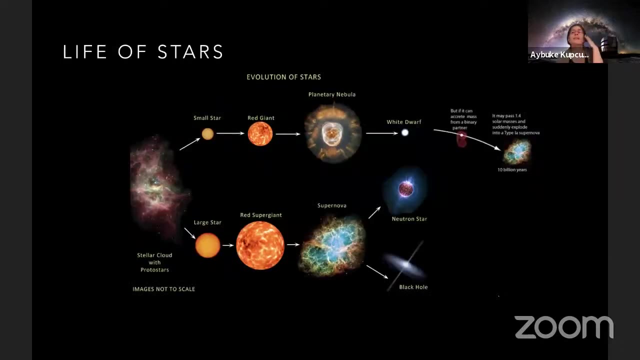 Or right after, basically during the optical afterglow phase of the gamma ray burst for the long duration gamma ray burst for some of these. So I'll just open a parenthesis here to tell you what the or to remind you basically what supernova is. 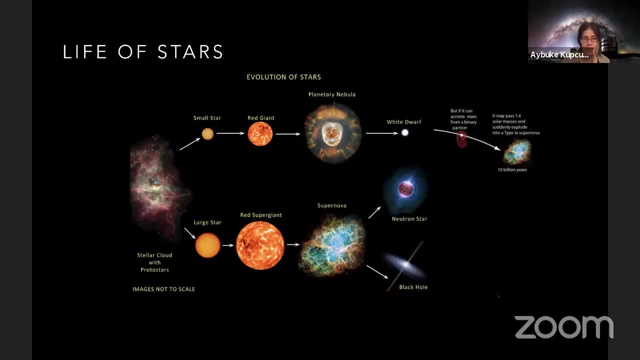 And so when we have a look at the life of the stars, so for most of the stars right, there are some very small or giant exceptions, so there are like two main parts of their life cycle. They start as a small star, like our sun. 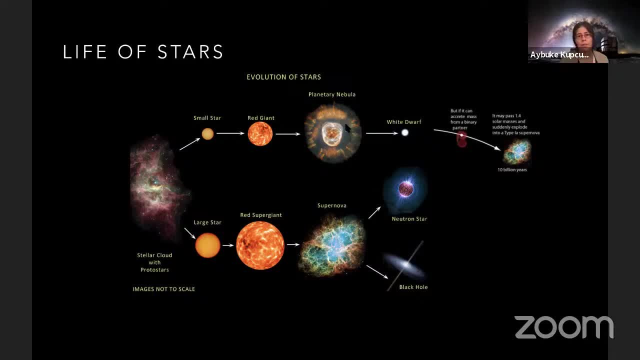 and turn into a red giant, then turn into a planetary nebula and then become a white dwarf. And if this white dwarf has a partner, if it is a binary star system, basically it can accumulate. the white dwarf takes material onto itself from its companions. 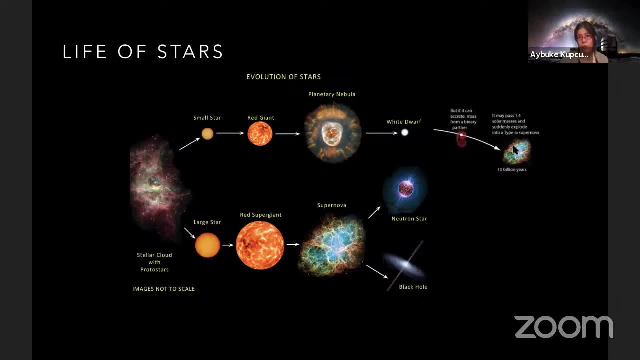 So it can form a supernova, and then it can form a black hole, and then it can form a neutron star, And eventually there is what we call a type 1A supernova. Basically, it explodes, leaving nothing behind, Whereas for bigger stars it's similar. 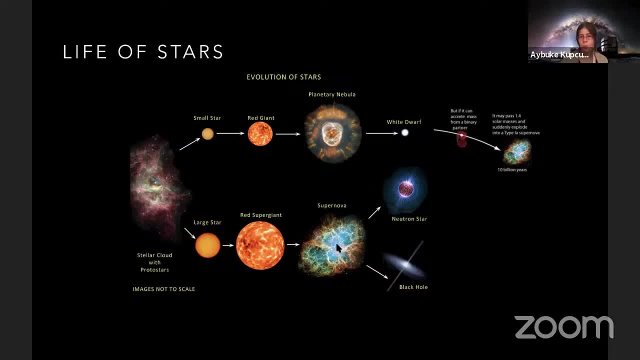 It turns into what we call red supergiant. but then after that there is the supernova. what we call core collapse supernova happens and leaving behind either a neutron star or a black hole, this core collapse supernova, um, sometimes together with the gamma ray, bursts the long duration gamma. 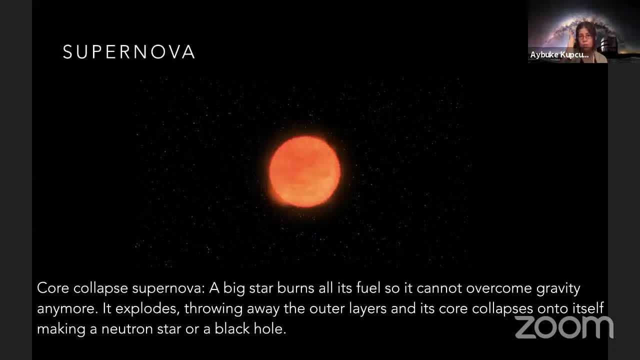 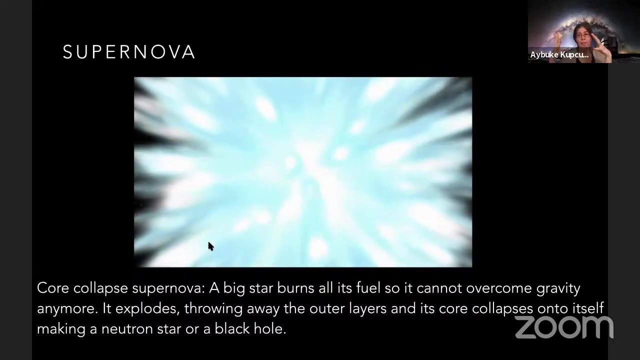 ray bursts. so this is a short video, um, it's just an animation about the core collapse supernova, but it's basically when the when these big stars um burn all of its fill and at the end there is nothing left to overcome the gravitational pull. so it explodes and throws away all the outer layers. 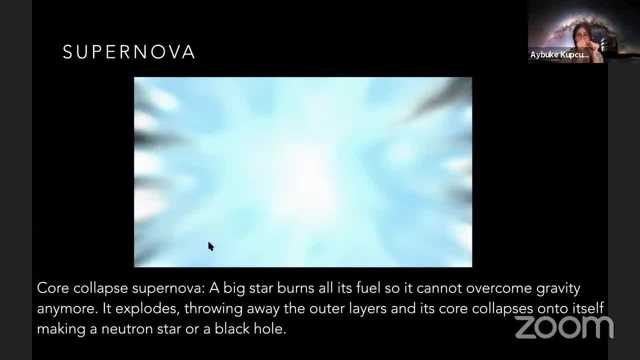 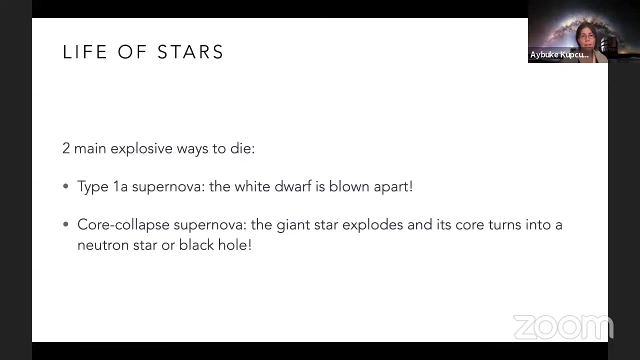 of the star, but the core of the star, and then cannot overcome the gravity and basically collapses onto itself, making either a neutron star or a black hole, depending on the initial mass of the star. so, as we knew, there were these two main ways, explosive ways to die. one is the when the white dwarf has a companion star, and 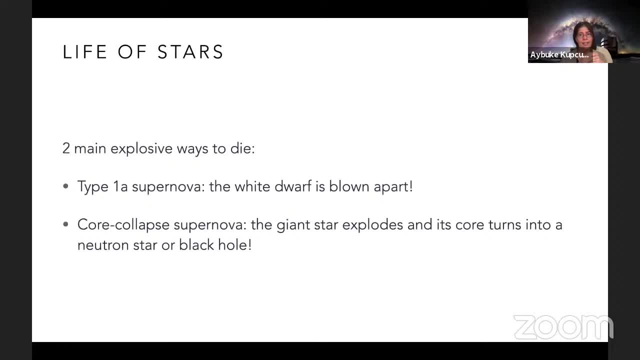 then it accumulates so much uh material that it just explodes and um blowing apart with nothing left behind. and the other is this core collapse supernova when the giant star explodes and its core turns into a neutron star or a black hole. but then when we um observe more and more gamma ray. 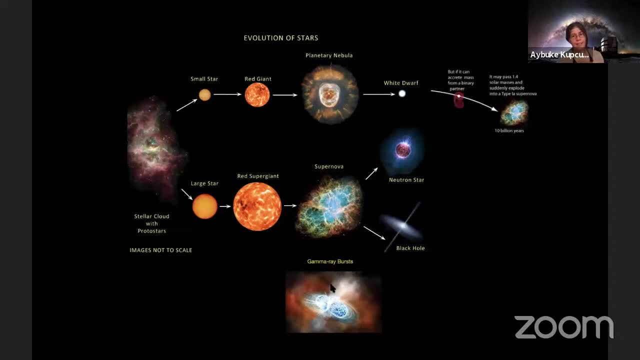 bursts, we realize that there is an another event happening for some of these large stars. so when? if the star um, as far as we can predict from the observations, if it is a very large one, like 30, 40 times the um, the mass of the sun, um, and if it is uh, if it has some, uh, other additional properties? 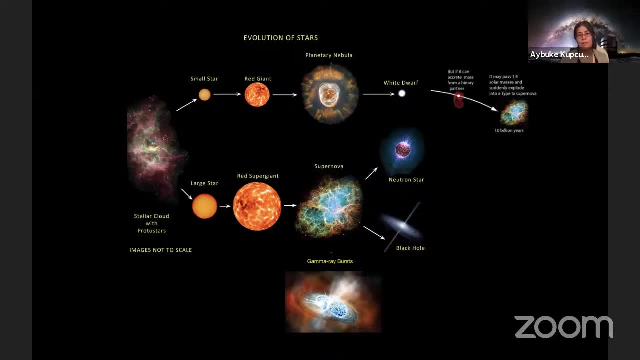 it can not only produce this supernova at the end of its life cycle, but also this gamma ray burst which is like uh again throwing jet um, like uh material its outer layers, but this time in a jet in the two directions and much more actually powerful than the supernova explosion itself. so 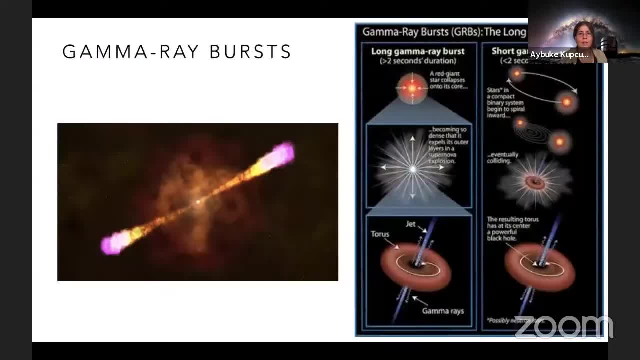 it's much brighter and much more powerful. so, yeah, this is, uh, basically what we know about camera. so, and, as i said, the short and long division is not just the duration, um, but the other properties which we um then know that the long duration gamma ray burst, the long camera verse, um, as i said, is. 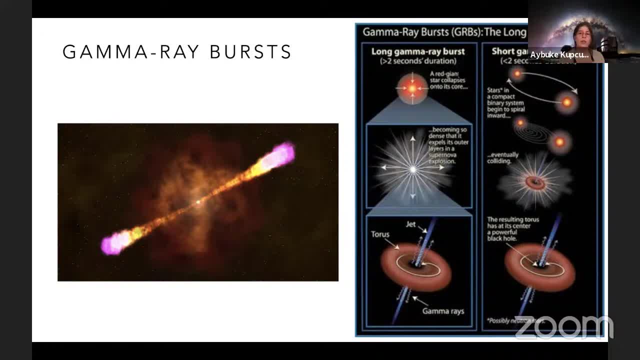 these massive stars, these giant stars collapsing onto itself and then basically throwing the outer layers in a jet, and the short duration gamma ray bursts are actually binary stars. and, uh, these binary stars, um, eventually, the, the, the two neutron stars, or a black hole and a neutron star, basically, and and they eventually, um, um, get closer and closer and collide into each other and 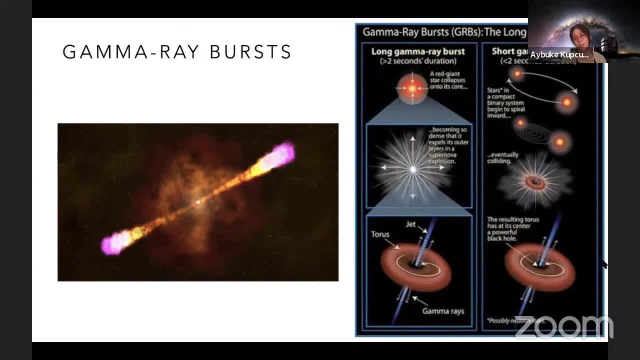 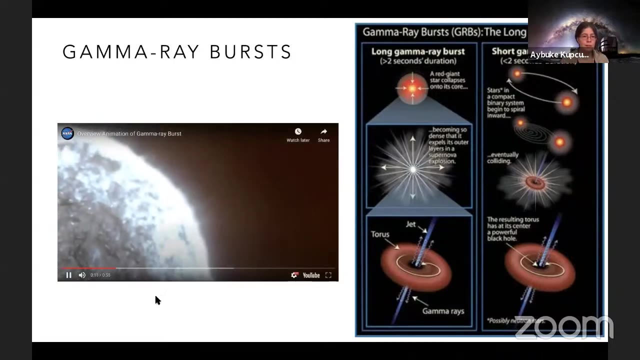 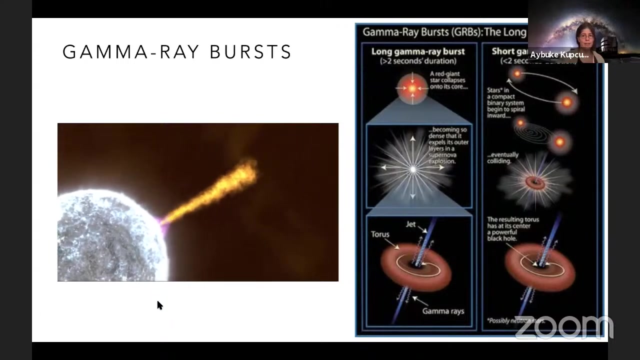 form- the um gamma ray burst, short gamma ray burst- and these are actually the ones that are also observed by the sectors. So yeah, this is a short animation about how this jet explosion happens. So we can see the big star And then it slowly starts to kind of throw the outer layers in a jet. 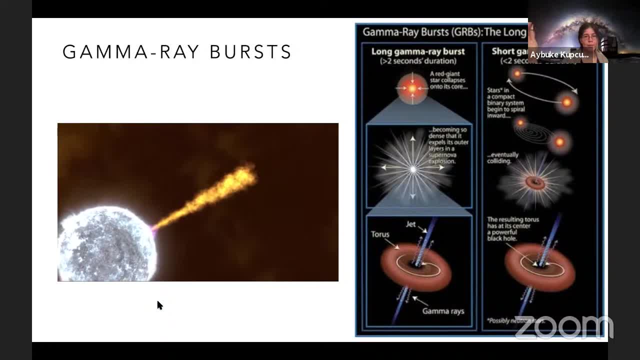 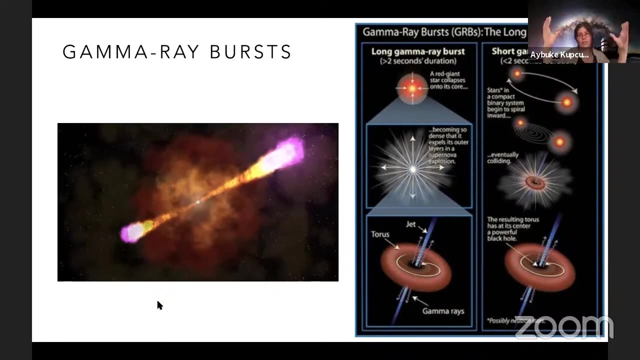 stream And then during that stream, there are some collisions between that material due to different speeds, which then forms the gamma rays and the afterglow, basically emission, once it collides with material right outside the star, the shell and the material surrounding the star. 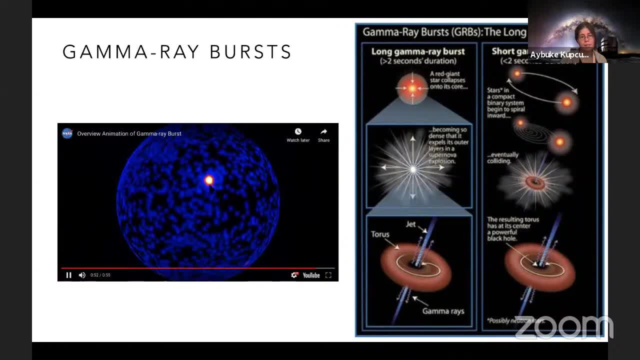 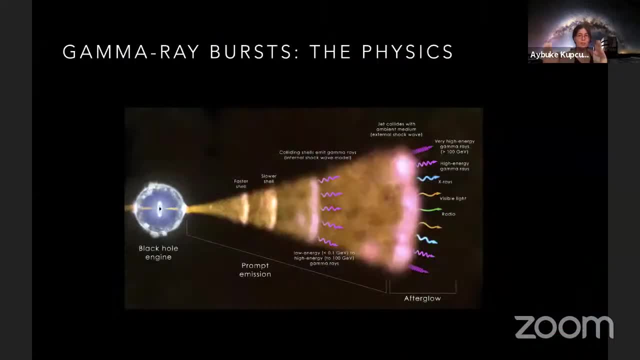 And then, yeah, we see it as a basically a big explosion in the gamma rays first. So this is the roughly the physics. obviously I won't go into the details, But, as I said, the gamma ray burst itself is due to the collision of the basically shock emission. 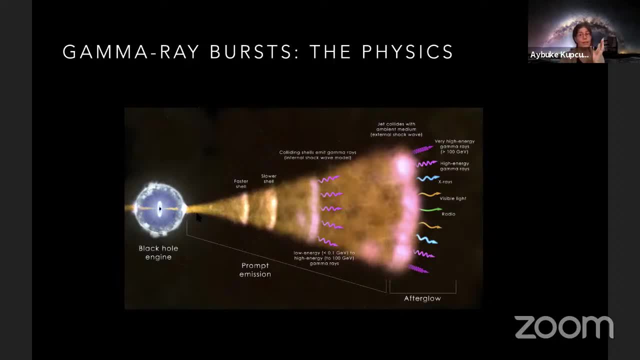 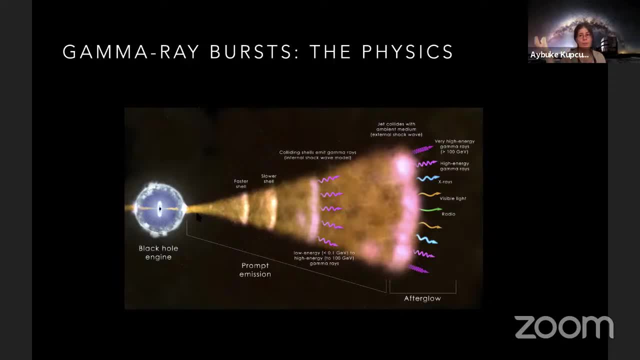 speed the material collides And then we see the gamma ray burst. And then, once it hits the material near the star, this jet, the ejecta, hits the material near the star. it also emits this afterglow emission in all the other light wavelengths. 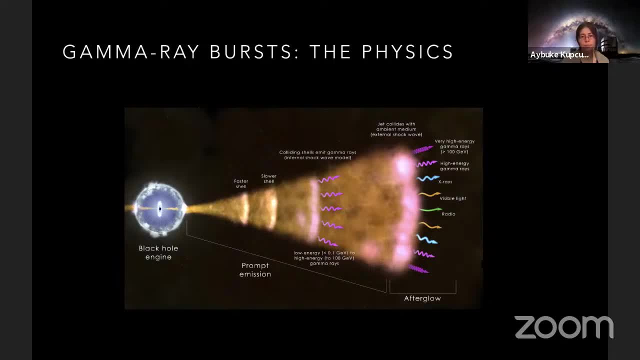 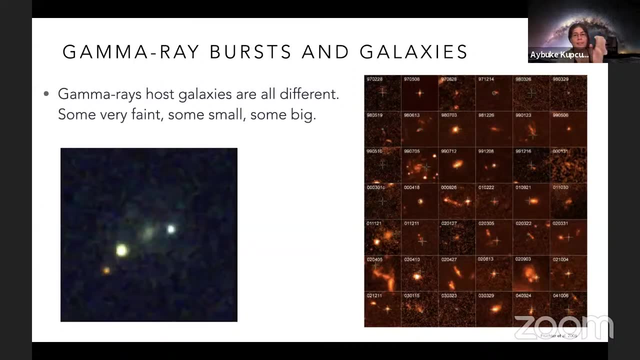 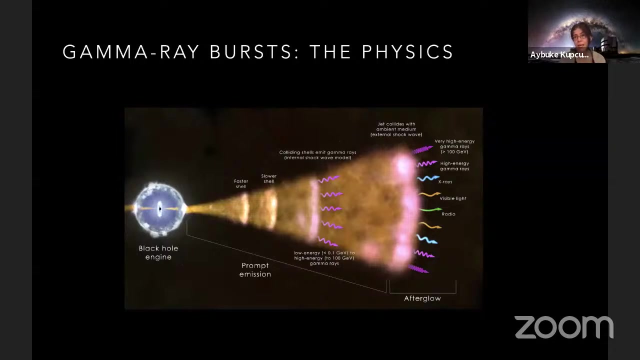 lighter and different energy light, from X rays, optical to radio, but that's not the only. i mean this is there is a lot of sort of interesting physics going on with the gamma ray burst. obviously they are the most energetic, most extreme explosions that single stars produce, and so they are very interesting laboratories of physics. but that's. 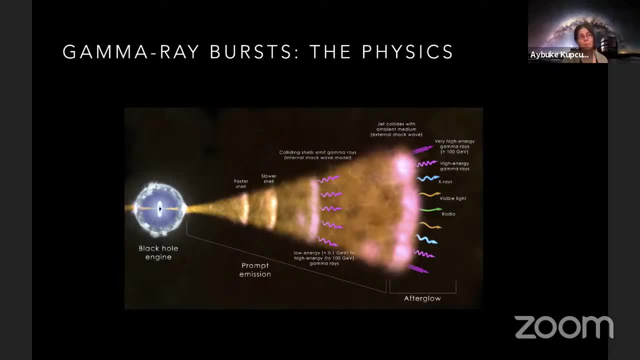 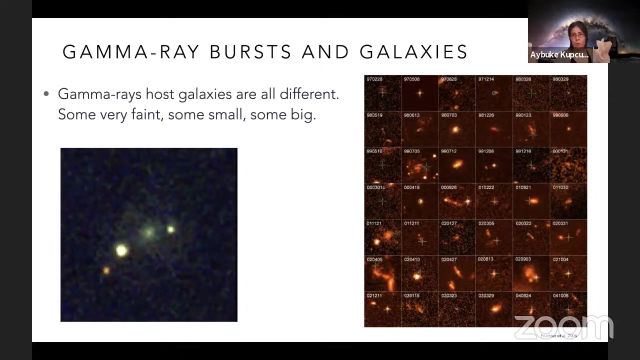 not the only thing that is interesting about them. so part of the title of my talk was exploring the universe using these deadly explosions, and the reason we can do this is basically gamma rays comes. we can detect gamma rays irrelevant of their distance to us, so i'll just come to that in a moment. but, as i said, gamma rays occur in. 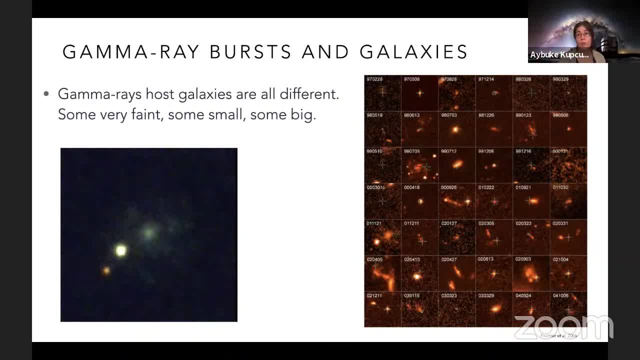 galaxies and once they fade away, we can actually observe the galaxy and get studied the galaxies. and here, actually on the right hand side, there are some images of different gamma ray burst galaxies- host galaxies, as we call them- and there are all types of galaxies: some are very faint, some are big, some are small, some 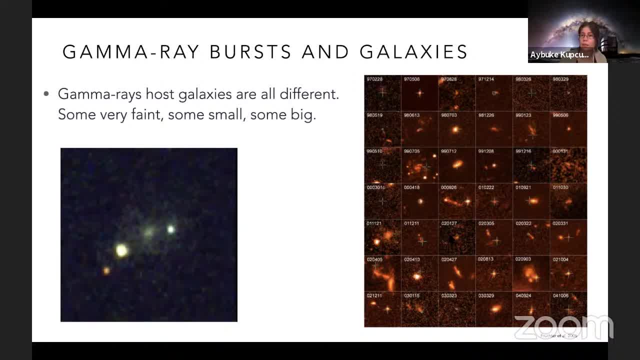 are irregular, some are spiral galaxies, like our milky way. so basically, um, they can happen more or less in any type of galaxy, which means we can actually use these gamma ray bursts to um to observe and and study um galaxy, the evolution of galaxies in time or or actually. 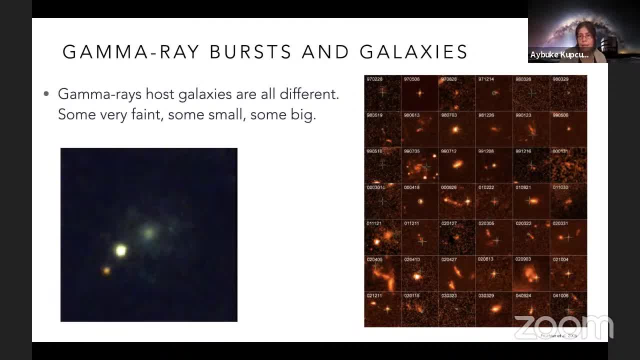 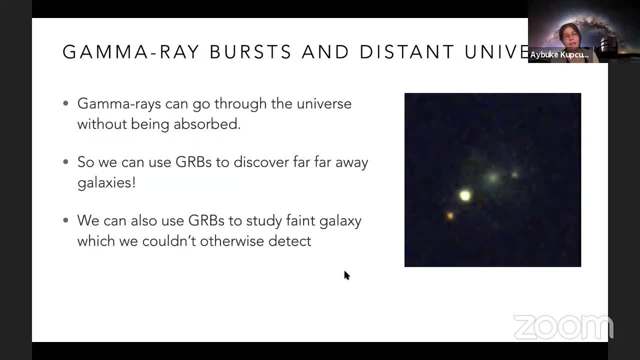 detect the faint galaxies that we wouldn't normally see in sky surveys um. one other thing is um, as i said, the gamma rays can go through the universe without being absorbed, which means that they can be very far away and we can still um see the gamma ray bursts, which is not the case. 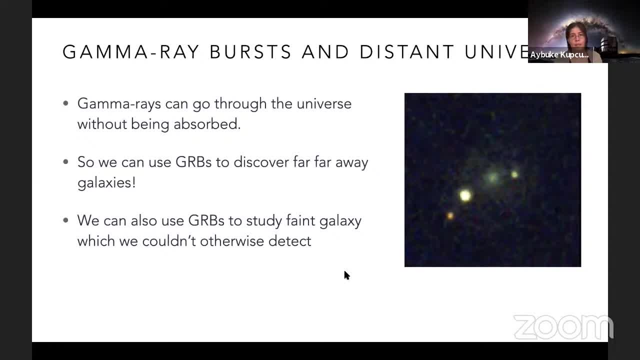 unfortunately for other wavelengths, mostly the in the optical and infrared the, the other galaxies in between us will absorb that and sometimes re-emit in in different light. but it means that we can actually see, um, everything, all the different wavelengths lights coming towards us. so we can actually use these gamma rays we can. so we can actually use these gamma ray bursts to. 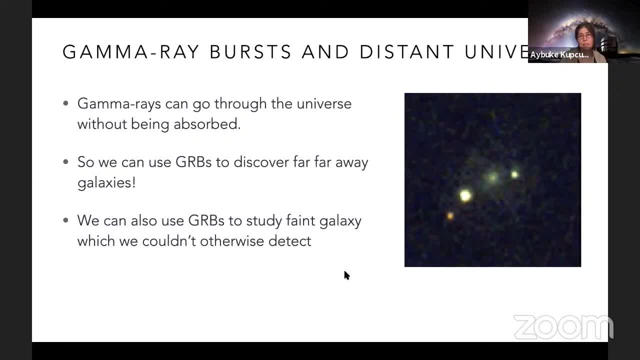 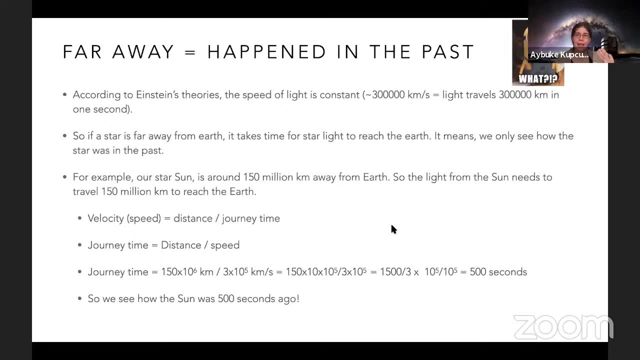 discover far, far away galaxies, um, and also, as i said, to study the faint ones that we cannot detect otherwise. so how can we do? this is um, so it's only not far, far away, but it's also. it means it happened in the past, because the speed of light is constant, so we can actually 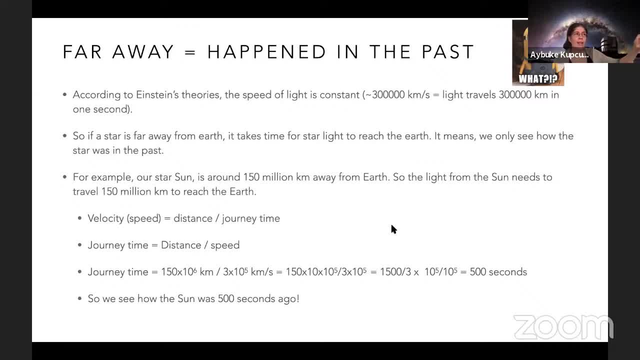 see galaxies that were formed uh, um much, uh long ago, actually, um closer to the big bang, much closer to the big bang, to the early universe, than us, and this is basically, as i said, due to the speed of light being constant. so i am just showing here um a very basic calculation, um, for instance, our 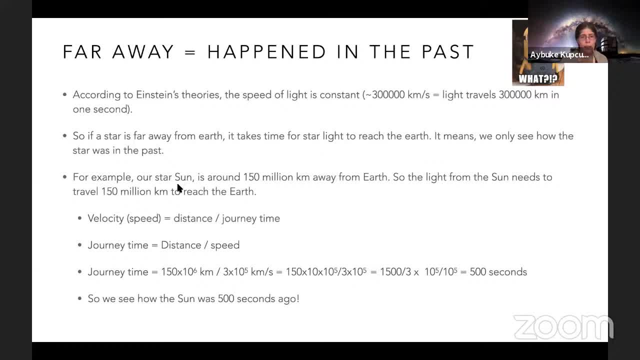 galaxy is very, very far away from us, and so we can see galaxies that are formed in a very, very, um, very, very, very uh dramatic way. so that means that, for instance, our sun, yeah, our star sun, is roughly 150 million kilometers away from the earth. so when the sun, when the light, starts its journey, 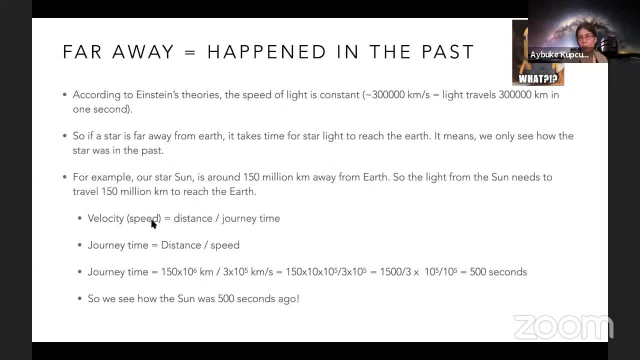 from sun to us. it needs to travel this 150 million kilometers to reach the earth and, as we know from basic physics, the velocity is the distance over time. so the and the time that this journey takes takes for that light that starts its journey from sun to reach us at Earth. 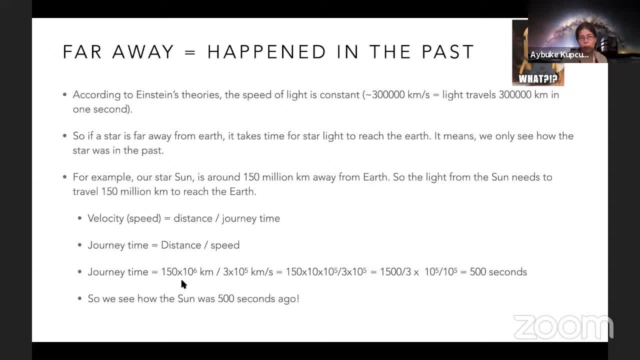 So it's basically the distance, which is roughly 150 million kilometres, divided by the speed of light, which is roughly 300,000 kilometres per second. So if we do this simple calculation, we find roughly 500 seconds. So when the light starts its journey from the sun, it takes 500 seconds for it to reach us. 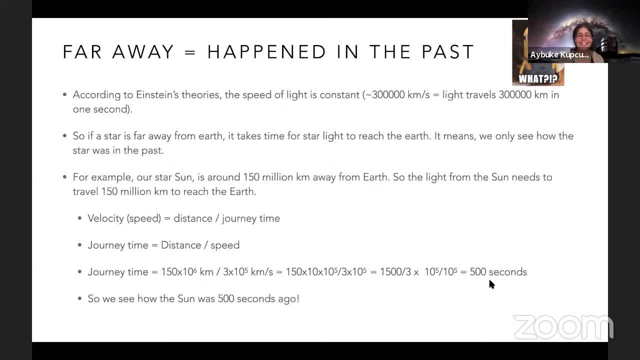 which is roughly eight minutes, And so think about much further away objects. So when a star is far, far away from us, this is, you know, like this is the nearest star to us, the sun- And these gamma ray bursts happen in other galaxies. 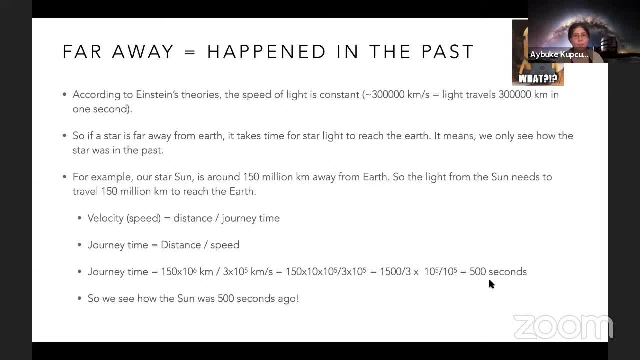 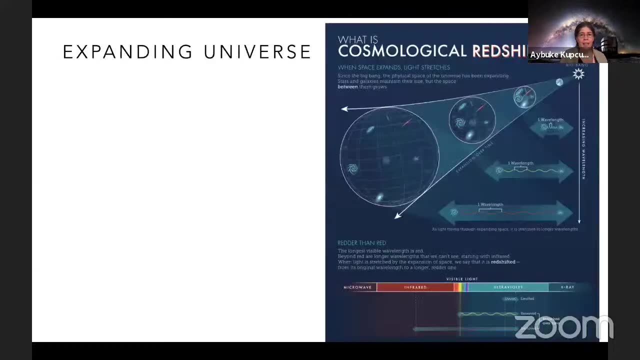 So you know we are talking about much further distances. So the light takes millions of years to reach us, which means basically we are seeing the universe when it was millions of years ago. So obviously for the universe the calculation of the distance is a bit more complicated. 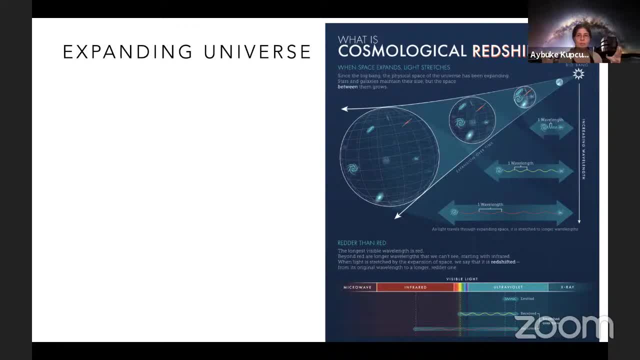 because, as we know, the universe is expanding, which means the distances actually increase. Obviously it's not constant over time. so it's not constant. So we have to take into account that calculation And also due to the Doppler shift. 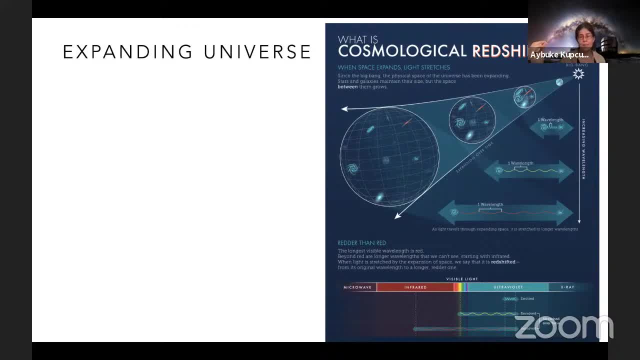 the light also changes its wavelength when it's. I mean, it starts its journey as a certain wavelength but then shifts to red before it reaches us because of the expanding universe. But so there is some additional physics going on, But the basic idea is: 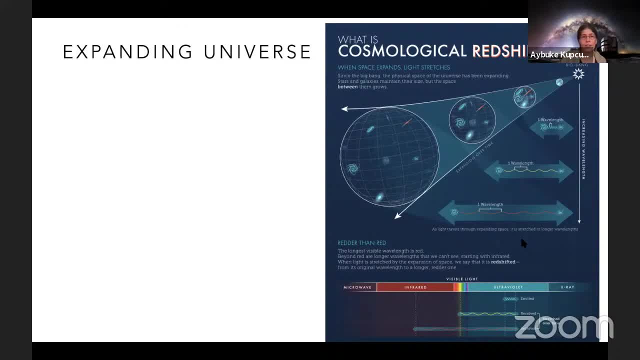 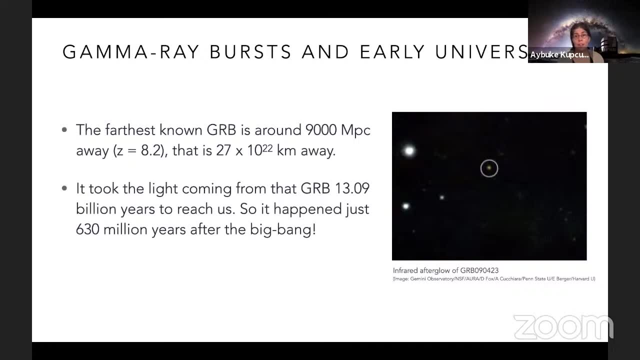 the idea is still due to the speed of light being constant, And so we can use gamma ray bursts, as I said, to learn more about the early universe, And at the moment, the farthest known gamma ray burst is what we call this cosmological redshift of 8.2,. 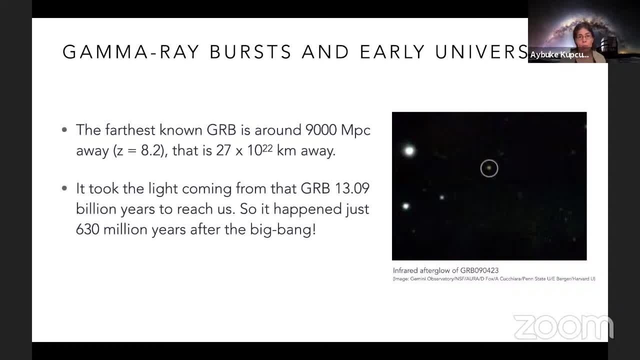 which is about 9000 megaparsec away, which comes up to roughly 27 times 10 to the 22 kilometer away. So yeah, I don't know if there is a name. I think the largest I know is that I want to want to go into the, you know. 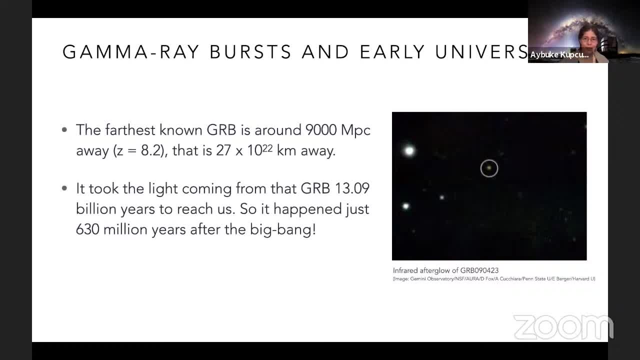 PETA or so. So it's, like you know, 10 to the 7 quadrillion or something kilometers away. So, and when we calculate this in terms of time that has passed, it's basically took light about 13 billion years to reach us. 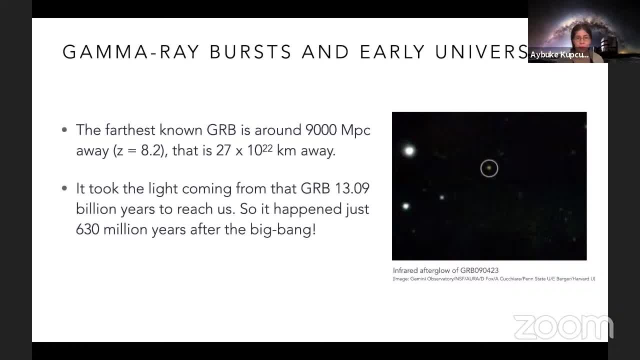 And so our universe is like 13.7 billion years old. So it's this far away gamma ray burst. here You can see the infrared afterglow of it has happened only 630 million years after the Big Bang actually. So there it is. 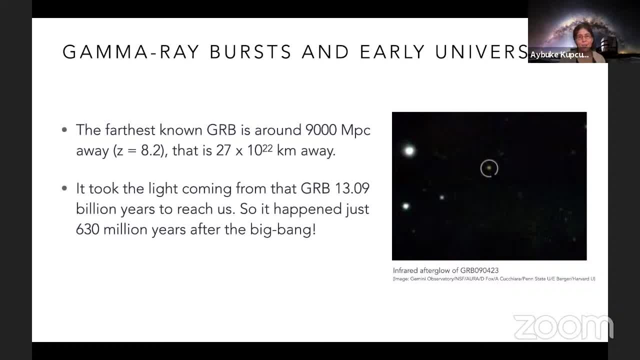 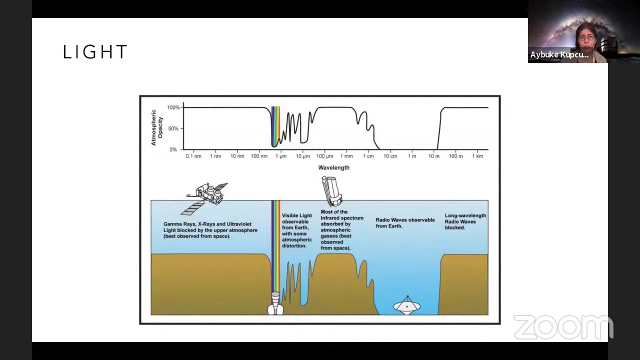 So this is really fascinating in that sense to be able to pinpoint these stars And sometimes, if you're lucky enough and have really powerful instruments, the galaxies that were among the you know first galaxies in the universe. even So, how we do it, I just want to spend a couple more minutes on how we do this, basically. 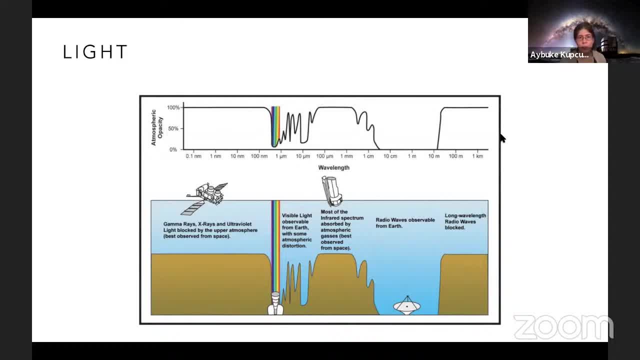 Yeah, So this is again the light spectrum, the electromagnetic spectrum, as I said. So we first observe them in the gamma rays. That is the one that can reach us without any problems. But lucky for us, for human beings and for the life on Earth. 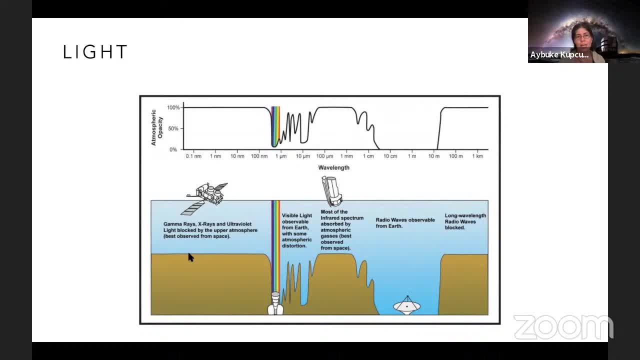 our atmosphere actually blocks the gamma rays and most of the X-rays and ultraviolet. So we have to use satellites, astronomical satellites with gamma rays And X-ray and UV, telescopes on them to be able to observe these And we can do optical and some of the near infrared observations on Earth, some of the infrared spectrum. 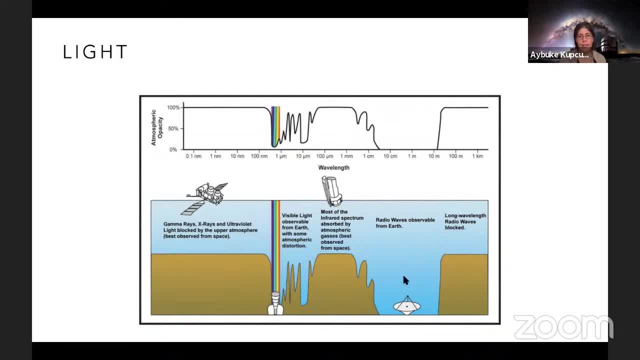 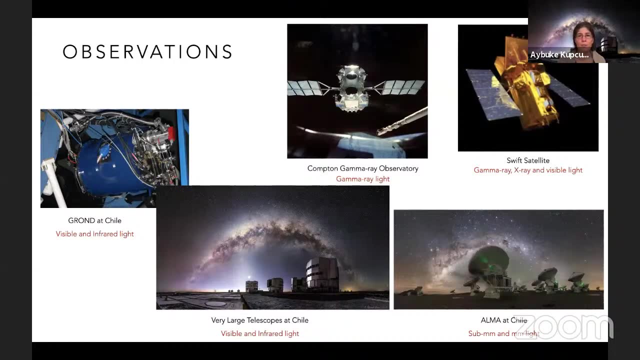 We again need satellites in the space, And then we can observe the radio wavelengths, the radio afterglow, for instance, on Earth as well, And so these are basically a few of the instruments i myself used for the um- gamma ray burst- research i did um. one is that um. 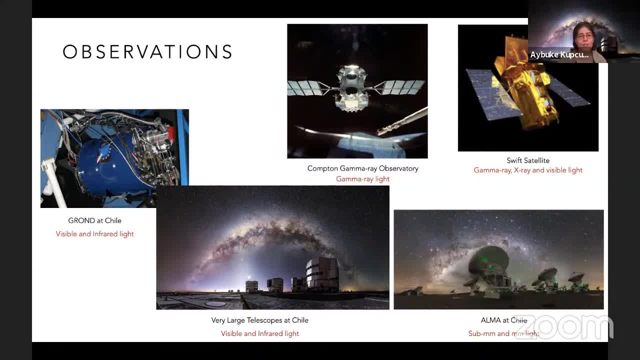 ground which was is now decommissioned, unfortunately, um. it is a visible and near infrared detector. it had, like uh. it was able to observe in seven um different uh light wavelengths at the same time, and this was mounted on on chile. as i said, this is the 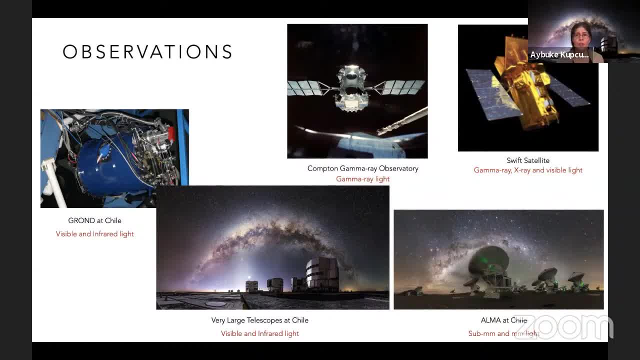 compton gamma ray observatory, which was the first one to um observe the um the x-ray afterglow of the um gamma ray bursts, which then meant we could learn much more about them, and uh, the current uh swift satellite and neil gary's with satellite. 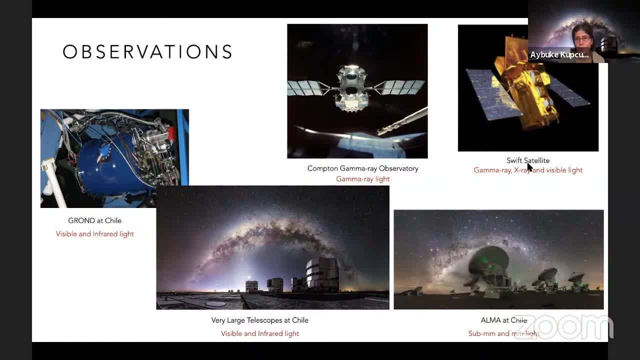 is the one um that is doing gamma ray, x-ray and visible light observations. this was particularly designed to observe gamma ray bursts and their afterglows, and you can see my virtual background here, the very large telescopes in chile. and again, these are, you know, used for many, many purposes. but 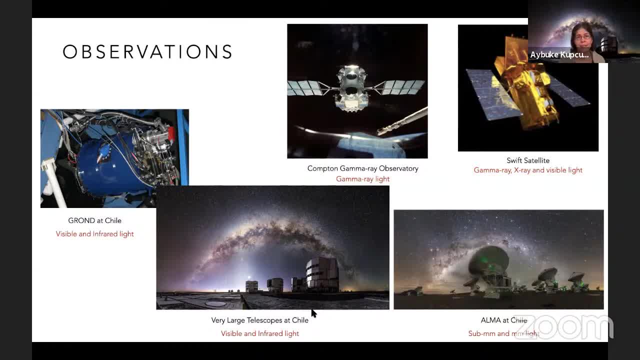 we used them to study the galaxies that um hosted, grbs camera reverse and visible and infrared light. and this is again um in chile, the alma telescope array and this is the sub millimeter millimeter observation close to the radio wavelengths. um, but yeah, and there are many. 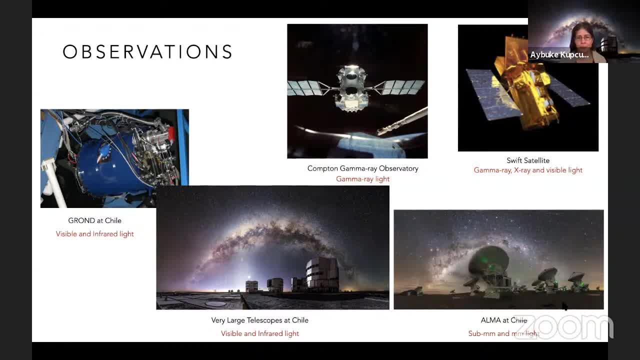 more, many more telescopes and and uh satellites. but basically what you need for the gamma ray burst research is that to have a gamma ray satellite and an x-ray one to pinpoint the x-ray afterglow to, to use the x-ray afterglow to pinpoint the location of the gamma ray burst. 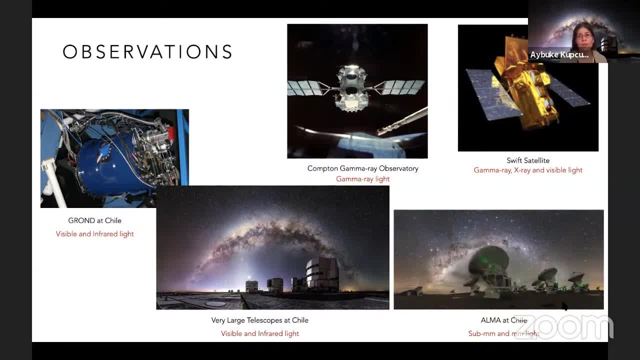 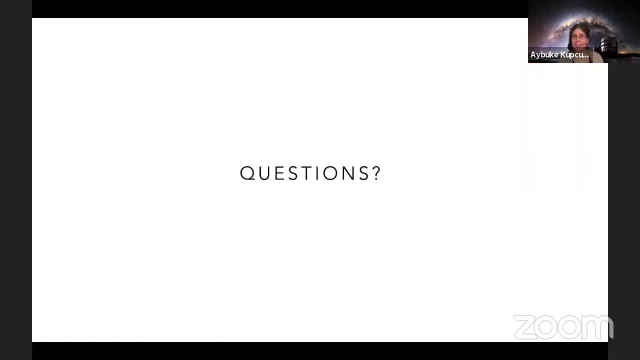 and then we use the telescopes on earth, big or small, to study the further properties. and i think that's it from me. any questions? wonderful, uh, thank you so much. uh, okay, that was absolutely wonderful. um, so there are some questions coming through. i'll say to anyone that has not asked a question yet: um, if you stick the, 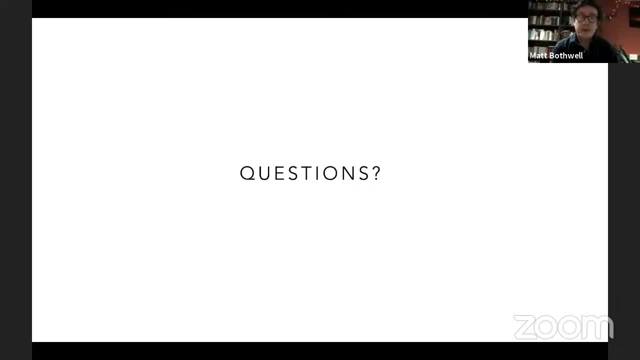 question down there in the youtube channel. i will make sure, um our speaker will get to it. um, so, um, going from the top, uh, someone uh would like to know. um, and feel free not to answer this, because i know you didn't mention this during your talk. 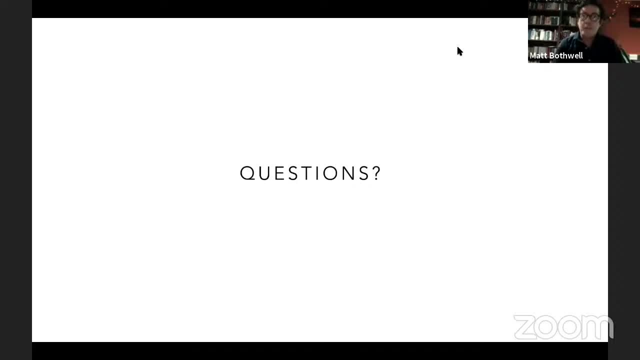 but about, um, cold spots in the cmb, and what might that mean? uh for uh, i would have loved to answer that, but the cosmology is not my area of expertise. i would you know, like, uh, i don't think. um, no, that's fine if you have any thoughts on it, but, yes, no, it's not my area either. right, i wouldn't have. 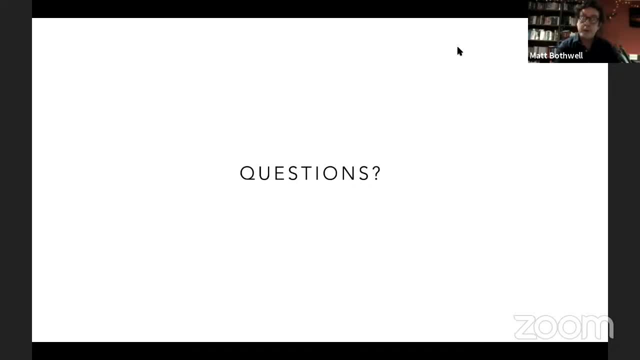 um. so we do have a question from wayne underwood, um, who was fascinated by the idea that when a binary system goes supernova, there's nothing left at all. so does that mean that all of the matter gets converted into energy? yeah, so it's not all binary systems. to clarify that, sorry. 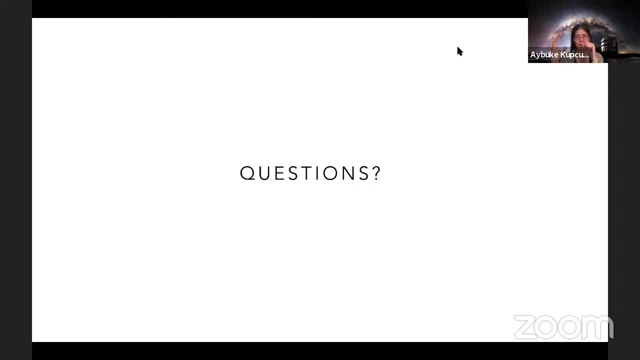 it's only when it's the white dwarf and and the normal star, basically, um, and eventually the, the white dwarf accumulates the matter and a certain amount of matter and there are other physical processes. but basically, yeah, it all explodes and converted, is converted into energy and there is. 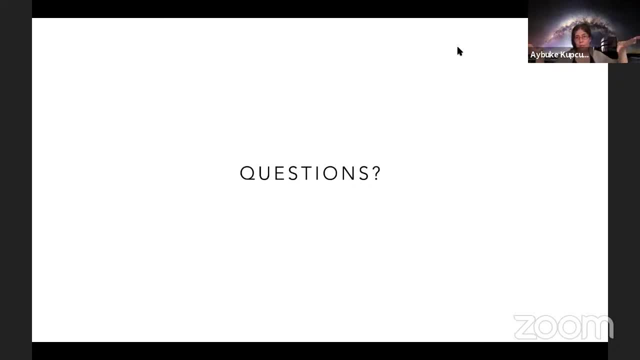 some- um, sometimes the nebula, some matter lying around, but there is nothing resembling a star, or no neutron star or even a black hole left. i mean, that's just an enormous amount of energy, right? just yeah. yeah, supernova, type 1a supernova- are very powerful and and they have also. 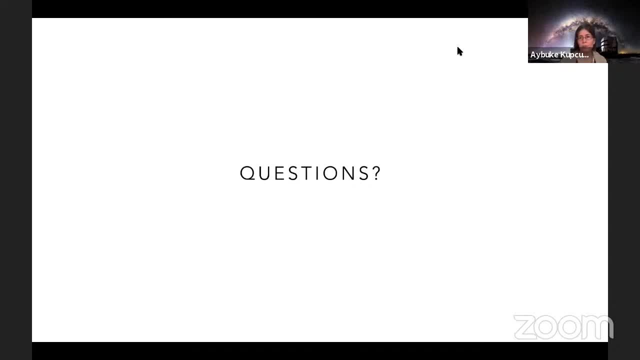 um, some certain properties that enables us to use them as- uh you know- candles, basically to, um, study cosmology. um, a question has come through which i think you did mention in your talk. maybe you just remind us. uh, what is the largest redshift of the gamma ray burst that we've observed? 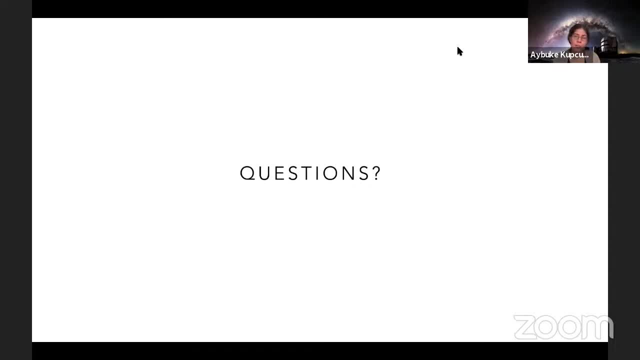 yeah, so the the largest one we know that is being com. that was confirmed spectacularly, spectroscopically, and so there are different ways of measuring redshift, and the most secure way is the spectroscopic redshift where we can um see the light in much more detail in in small. 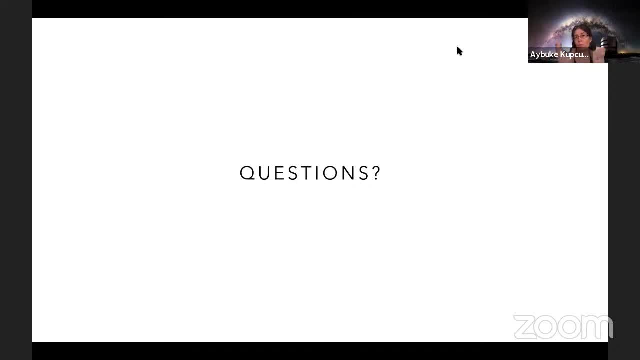 bins of small sections of wavelength. so we we know for sure where it is coming from and it's it properties basically of the um, of its source. so the the largest one that is confirmed in that way is the 8.2, the grb 04090423, i think the gamma ray bursts are named. 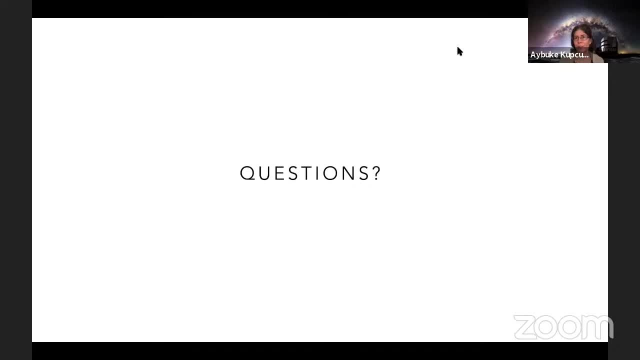 um by the date they happen. so, oh, 90423 is the 23rd of april 2009. yeah, and there are some um other grbs. there is a redshift um bigger than nine one, but unfortunately that was only the redshift was only calculated photometrically. um, but it's a redshift that was only calculated photometrically. 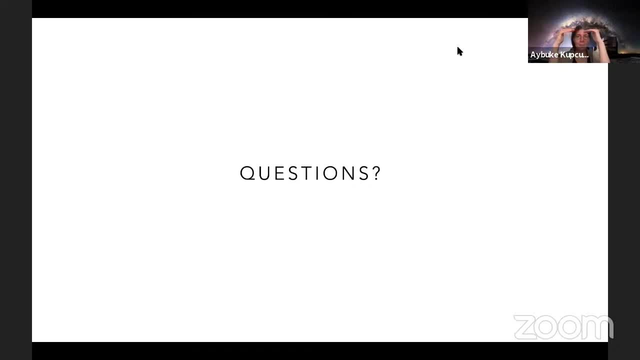 which is um when you don't, when you see um the light in certain filters like infrared, and then you don't see anything in the optical for instance, then you can roughly estimate the redshift. excellent, thank you. um. i will say there are lots of comments coming through saying they very much. 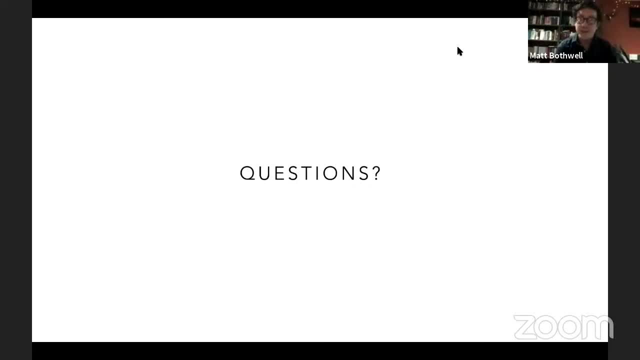 enjoyed your talk and they enjoyed the way you presented the spectrum. people found it very nice. um, can you talk at all, uh, about whether gamma rays might have an effect on the weather here on earth? oh, yeah, well, i mean, um, so these ones that are basically what we call cosmological, they are 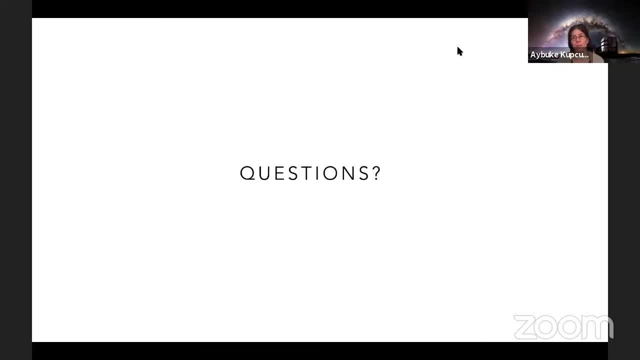 happening in other galaxies, um, and which don't have any effect on us, so that it has to be quite nearby to um to have the effect on our atmosphere. so far we haven't detected any in our galaxy, which is possibly a lucky thing, but i mean um. 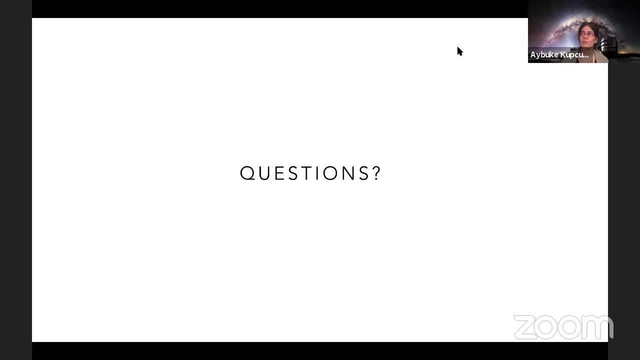 uh, again to, apart from, i would say, um, small disruptions, it wouldn't have any major effect unless it is very nearby, um, okay, um. so a question from jessica, um, who wants to know about the redshifts. um, so, do the gamma rays get redshifted as they travel through the universe? um, yes, but uh, because the 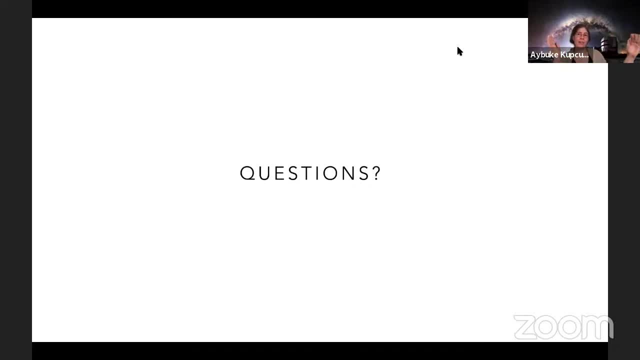 what we call gamma rays is basically a very, very um large portion of the electromagnetic spectrum spectrum, the light spectrum. their redshifting doesn't affect that much, So what we use to measure the distance of these stars is usually the visible and infrared light, because we 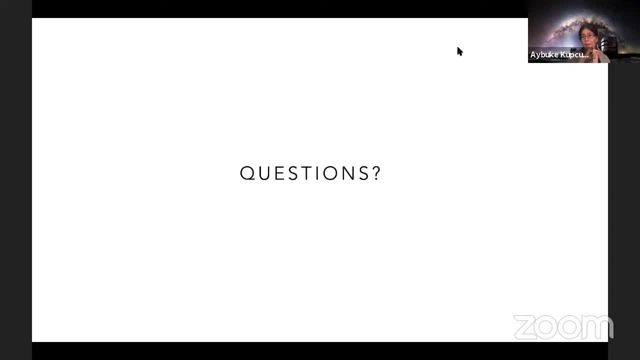 can observe the effect of the redshift much better there, And also because we can- I was saying this word spectrum- we can have a much more detailed spectrum. So see the light coming from, you know like with individual energies or wavelengths, in much more detail than in. 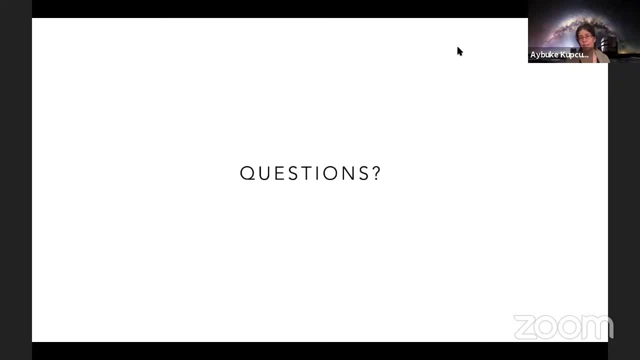 gamma-ray bursts. So in visible light and in infrared we can see these in much more detail. So that's what we use to determine the redshift, hence the distance. Wonderful. So there are questions coming in thick and fast. Are you okay to stay and answer? 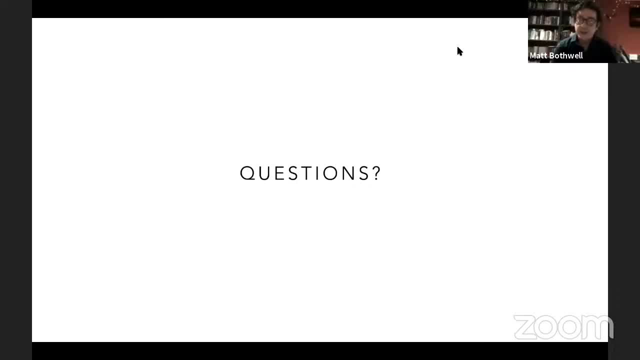 Yeah, yeah, yeah, I'm happy to. So, Sylvia would like to know: how much more do you think we have to learn about gamma-rays and gamma-ray bursts? So I mean, there are certain aspects of them, for instance, some of these short duration gamma-ray. 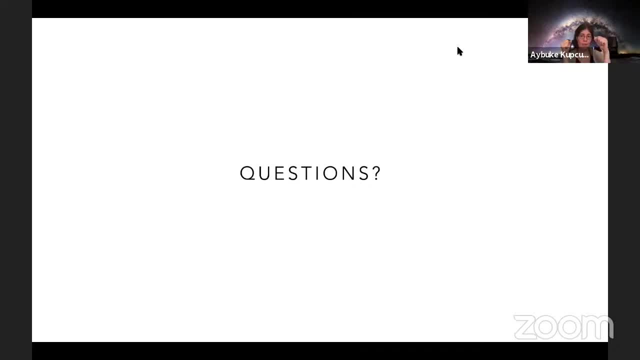 bursts that are shorter than two, Some are longer than two seconds. that we think are due to binary star, to neutron stars, For instance, the collapsing into each other. We see, for instance, from some of them now, thanks to LIGO and Virgo, we see the gravitational waves. So these two coming together gives us much more. 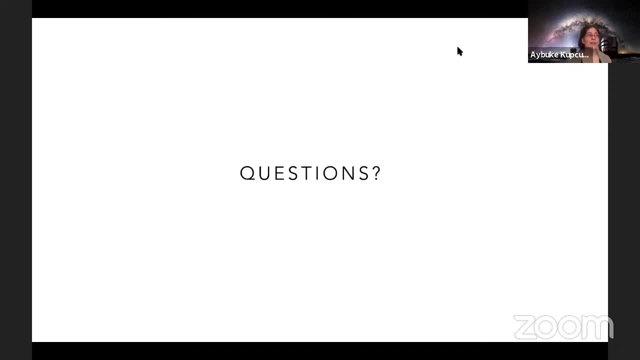 information about the physics. Some, for instance, are thought to be connected to now what we call soft gamma ray repeaters, which are actually a single very high magnetic field- neutron stars that regularly emit in gamma rays, And there is some indications that some of these short DRVs. 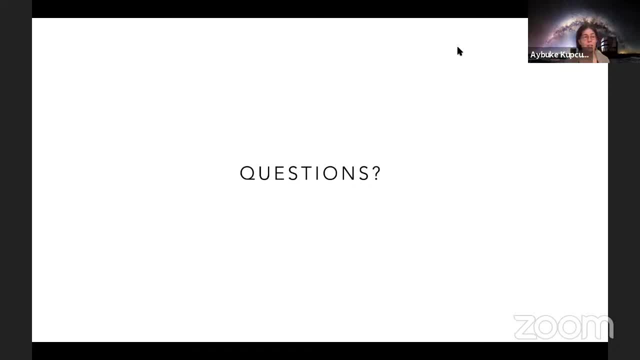 can be actually these repeater stars. So there are still unknowns in terms of the gamma ray bursts, what they are and how varied they are. But, as I said, there is also another interesting aspect: that we can use them to study other galaxies and to have more information about the early universe. 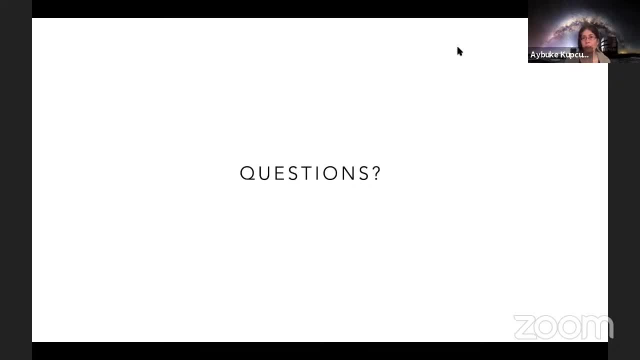 to pinpoint the first galaxies and to study them. Thank you, A question from Richard, who would like to know how common are gamma ray bursts really? Because if we see them, this narrow jet has to be pointed at Earth. Yeah, yeah, yeah, That's a good question. I don't know the numbers off the top of my head. 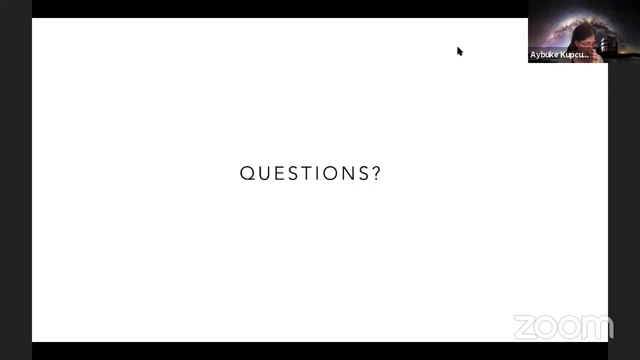 because it's been a few years that I have done active research in this field, But I remember that I think, for instance, Swift satellite detects around 150 DRVs per year, So we can calculate from that, like the galaxies That are roughly around, and then we know that, the angle of the jet from that, So, which is usually 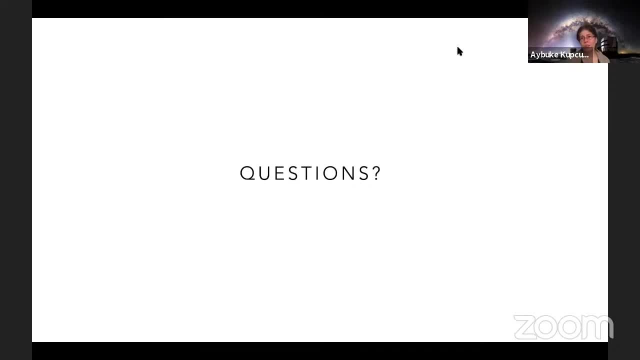 smaller than 30 degrees. And so, yeah, I mean they are not very rare But, as as Richard said, due to the jet nature of the emission, we don't necessarily see all of them, unfortunately. I'm going to, I'm going to ask a question that I know, I think I 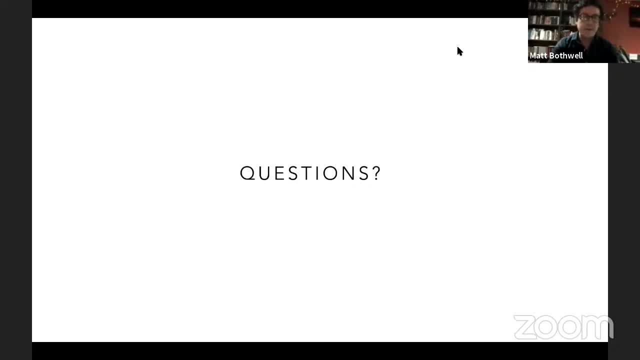 know is a challenging question. Someone wants to know how is. are the jets formed? Oh yeah, good question. It's mainly due to the spin. basically is angular momentum. So one of the requirements for these gamma ray bursts is I was saying they have to be very massive And they 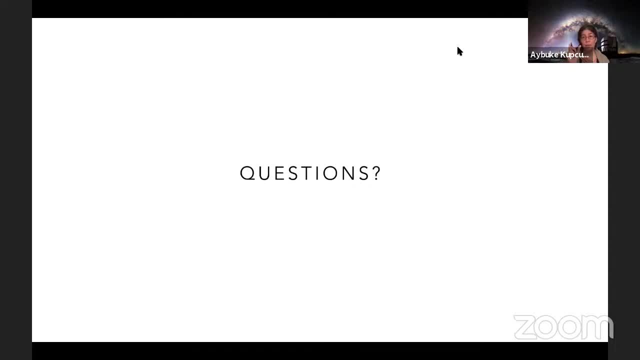 need to be low metallicity because they need to be spinning very fast, So they need to conserve their angular momentum through their lifetime, And so basically, it's just the angular momentum spinning star. it doesn't just explode in all direction because of the spin there. the material flows away in the direction of the spin, the of the 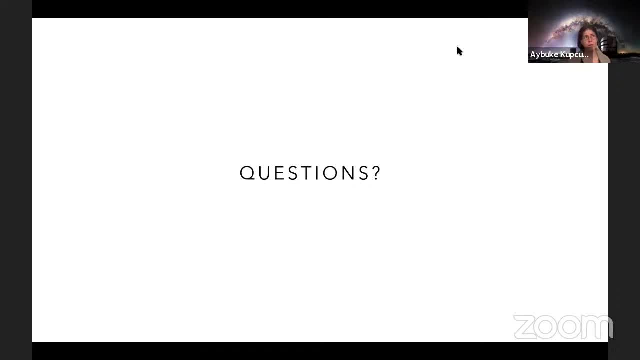 star spin, axis of the star, basically, Or Yeah, Thank you. Angus wants to know: is there any evidence that gamma ray bursts have ever caused an extinction here on Earth? That's a good question. I personally I don't know, But so we do know. as I said, 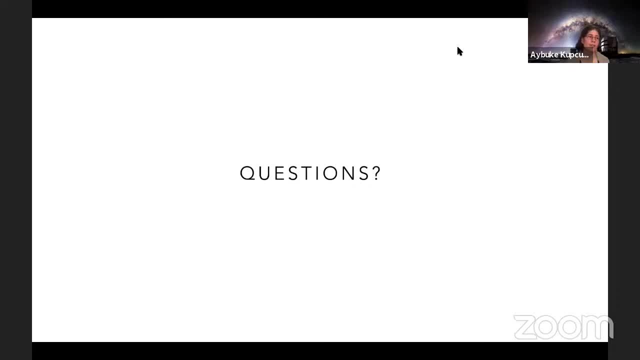 the properties of the well. but yeah, if it happens, what we could see would be just remnant black holes. So the thing with the gamma ray bursts, because once they happen, right after a few days you don't see anything anymore. So you have to be. 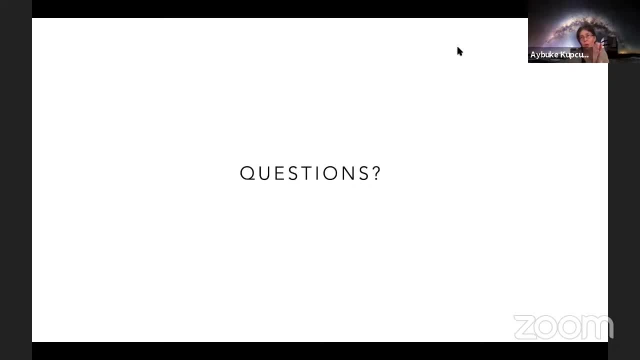 very fast. um, you know, point your telescopes, observe the thing and get as much information as you can, and then, if it's in another galaxy, then yes, you can observe the galaxy and study the galaxy, but for an extinction event it had to be very close to us, right? so it means that 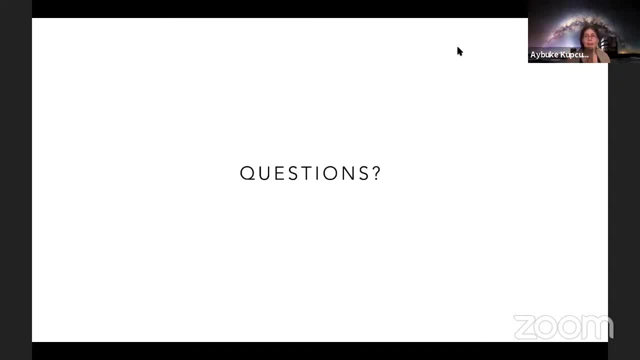 everything happens in a few days and what's left over is most likely a black hole. i mean, if it's a neutron star, again, it has to have certain properties, like uh, be a pulsar, for instance, for us to be able to observe, otherwise it has to be a black hole. and then, which means, you know, unless 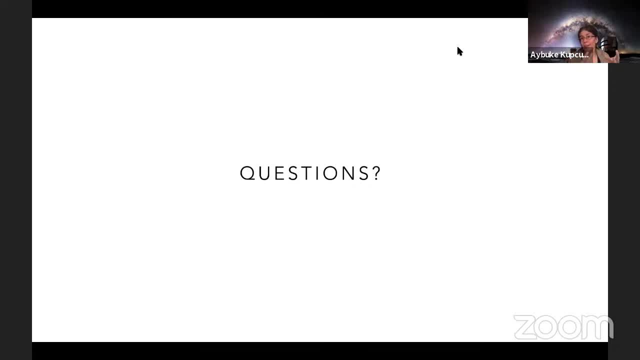 there is a, a companion star. we won't be able to see it, so it's really difficult to judge. uh, you know what could have been in the past in terms of the gamma ray bursts that are um near us? so yeah, i'm sure i've. i've. 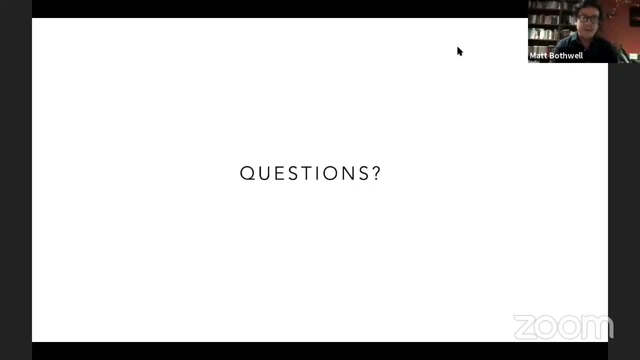 heard some theories, because i think the there was obviously the famous extinction that wiped out the dinosaurs about 65 million years ago, but yeah, there was an even bigger one about a bit more than 200 million years ago, and i've heard people hypothesize that. yeah, i mean, it is definitely. 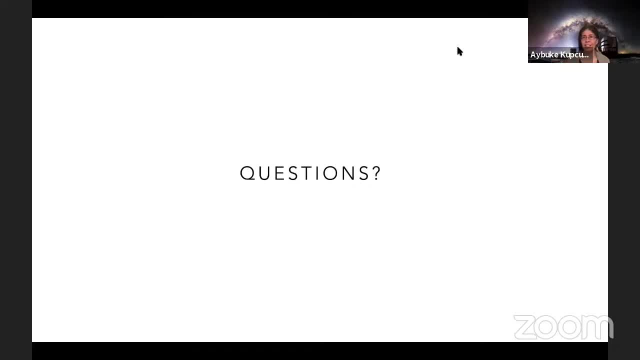 possible. it's just that you know, observationally it is not so easy to, you know, say, okay, i see there is a black hole, you know it might have, because, again, with, even with the black hole, even if you see a black hole, it could have turned into a black hole with just a super. 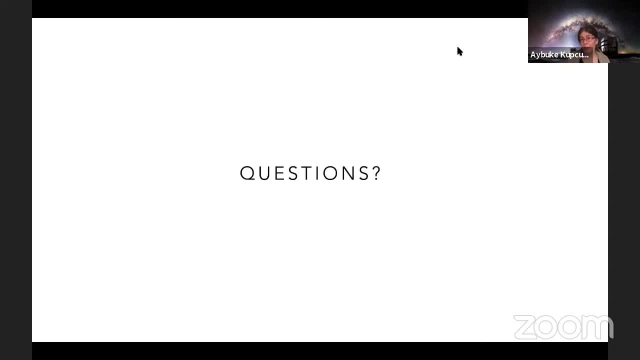 nova, uh, which is not as powerful as gamma ray bursts. so it's really, at this stage, it's mostly speculation, i would say, rather than you know astronomy. um, absolutely yeah. um question from dylan, uh, how big is the biggest gamma ray that we've ever seen? um, so i should say: sorry, i'm. 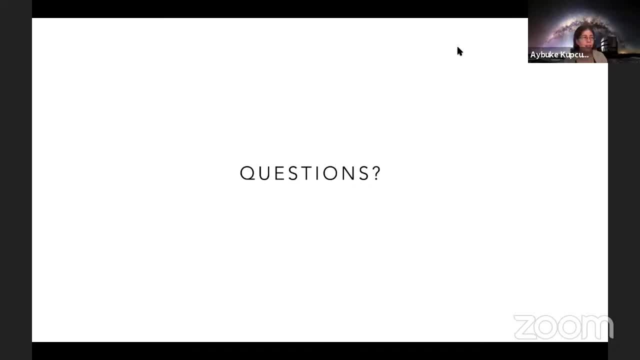 guessing it's in terms of the energy. so these are like um hundred and sorry, um ten to the fifth, to ergs, so they're really really very powerful. i don't know off the top of my head how i can convert this into something that makes sense to non-astronomers, but, um, you know, they're. 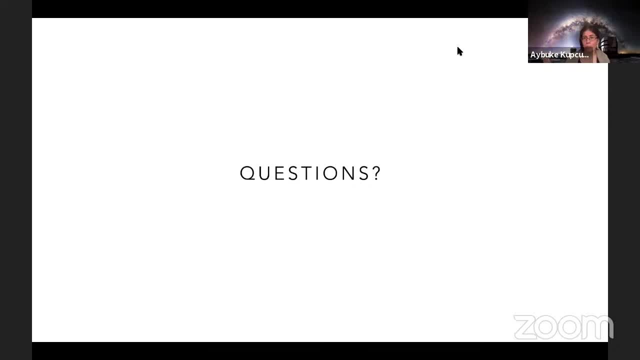 like uh, hundreds times more powerful than supernova, which are very, very powerful explosions, so um, and the thing is the it's not only the peak energy right. so for, for instance, for long duration gamma ray bursts, it start, goes uh into burst and then it slowly declines, i mean it slowly fades. 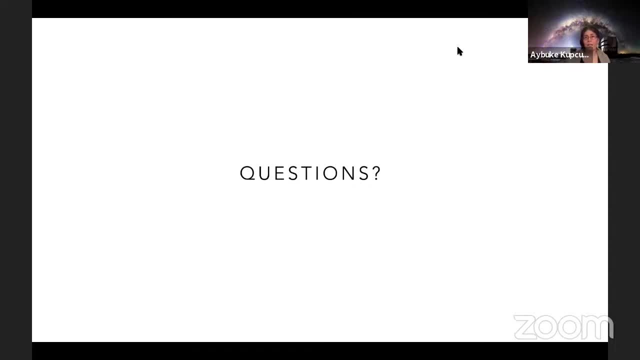 away, which means there is still a lot of energy in gamma rays coming uh, um, towards us from that source. so there is a lot of total energy budgets there, um, so i might. i might ask two or three more questions, if that's okay. the uh, everyone is saying this is a fantastic talk. i think you've 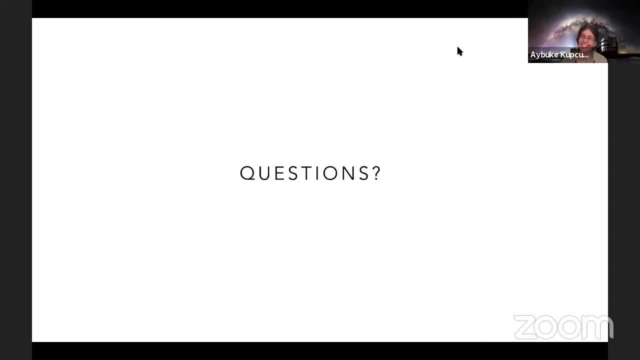 really picked there and dressed. i'm glad to hear that. um, scott armstrong would like to know which one is more powerful. is it the short term or the long term bursts? um, it is the uh. i would say it's the long ones. i mean the short. 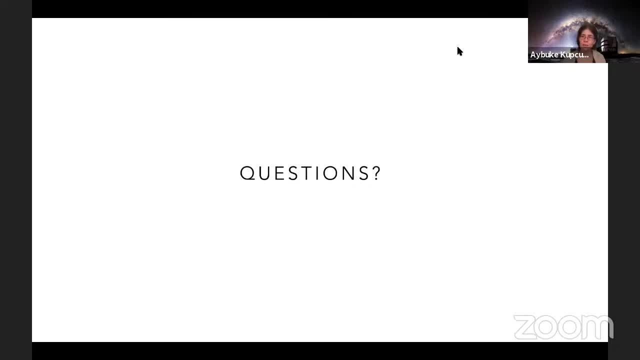 ones produce harder um gamma rays, so it's kind of more um high frequency, more energy. but because their um total duration is very, very short, shorter than two seconds, the overall um budget, energy budget, is not that high, whereas the longer ones- actually there are some that are um that took um several minutes. even so, um yeah, the the longer. 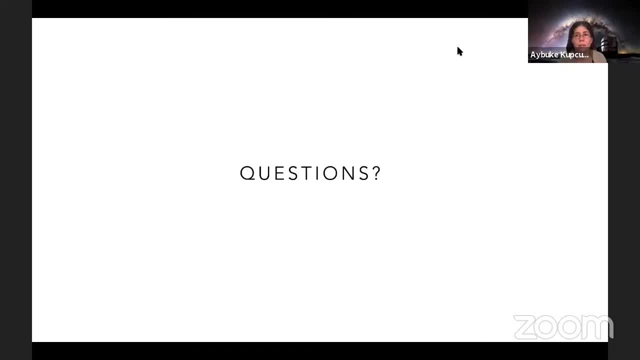 ones are, overall, more, more energetic. um, are gamma ray bursts predictable? um, yes, um, because from all these observations, as i said, we know that the the most likely source for the long duration, gamma ray burst are these, uh, very, very big stars that are spinning very fast and so um what we call wolf ray type stars. so we know, for instance, 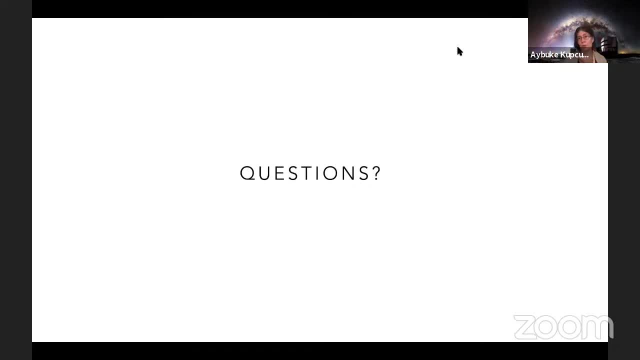 some wolf ray stars in in our galaxy which will likely to end up with gamma ray bursts, but it is a very long timeline, as everything else in in astronomy, even though the the burst itself is a very short event, the, the life cycle of the star that ends up in the short term bursts is a very 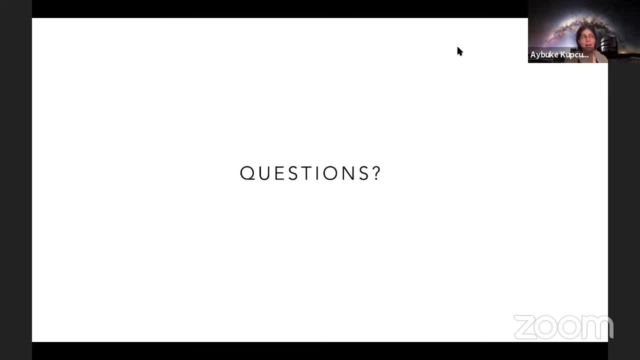 with the birth is a very long one, and then, as I said, the short gamma ray bursts are the binary systems, which has a neutron star in a neutron star or a neutron star in a black hole, and we don't necessarily know all these because they have the. I mean, you cannot observe a 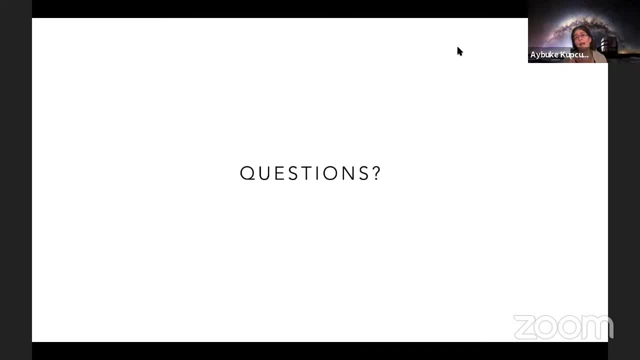 neutron star or a black hole, unless it is for the neutron stars. there are what we call pulsars, for instance, which are pulsating light in radio wavelengths, or some of them in x-rays and so on, which then you know, we know or otherwise. yeah, so we don't necessarily know which of these systems. 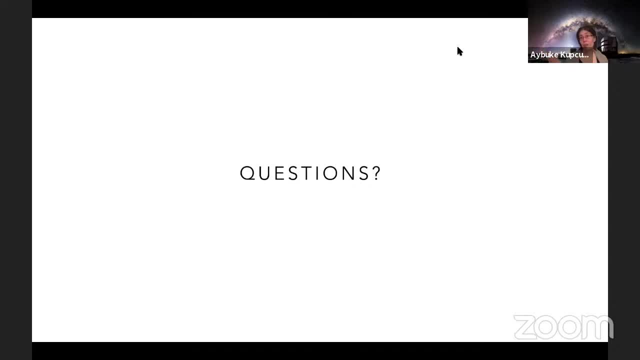 are in our galaxy, for instance? I mean in other galaxies. our telescopes, our technology is not good enough, unfortunately, to pinpoint the location of the individual stars, sure? so I'm going to make this the last question. I'm sorry there are questions coming in too fast to answer, but I'm afraid we, I think we need to give our 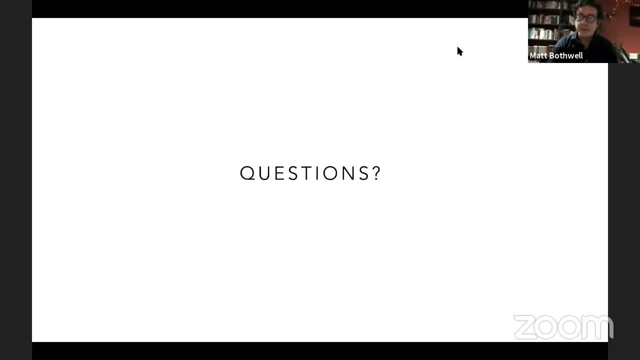 speaker a bit of a break after that fantastic talk. so the last question. someone would like to know a bit more personal, if you don't mind. when did you start studying astronomy, and what do you think might be the best way for some young people to start if they're interested in it? I have actually 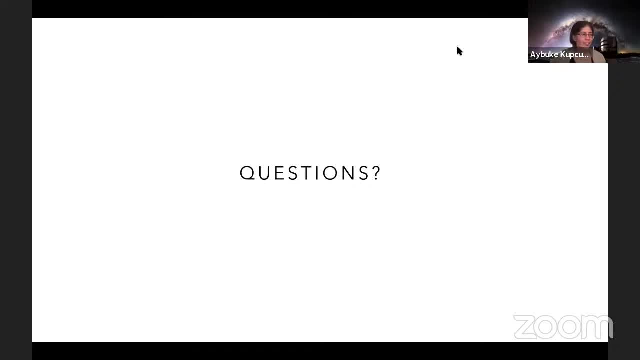 been interested in it for a long time and I think it's a very interesting journey in my career of as an astronomer. I studied physics, so I started studying physics in Turkey and I was actually more interested in, you know, like quantum, electrodynamics and that kind of or general 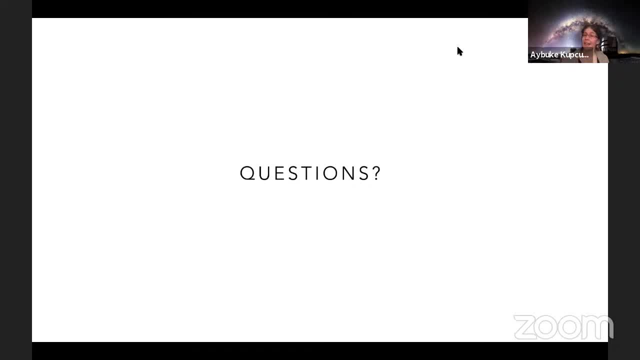 relativity or spring theory, type of more math, heavy physics. then I had a fantastic professor studying x-ray astronomy, and so it was the thing. I mean like I never had a telescope as a kid, so I'm really not your typical astronomer. but so I moved to x-ray astronomy during my master's and then 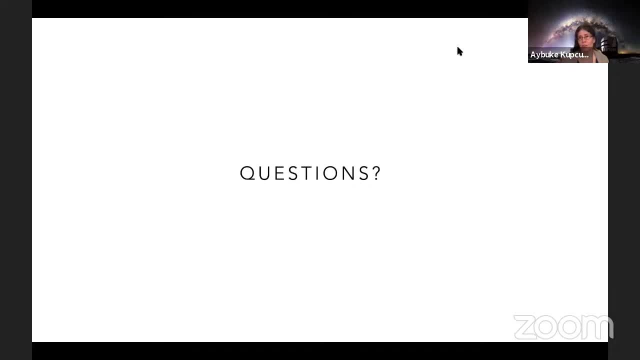 went to Germany and actually worked with this front instrument and started. so I was actually fascinated when I first heard about gamma ray bursts and and that's how I chose that in for my PhD subject and then eventually ended up here in Cambridge and doing other interesting things on top of those. so, yeah, I mean you know, like there are. 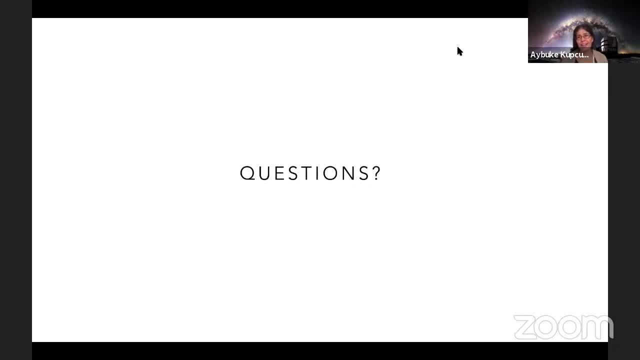 there isn't one way to, I would say, end up as an astrophysicist or astronomer, but like, if you really like it, want to learn more, you know like, start digging into it and start learning. so for observational astronomy, it's more: yeah, you need to know statistics, you need to know programming. 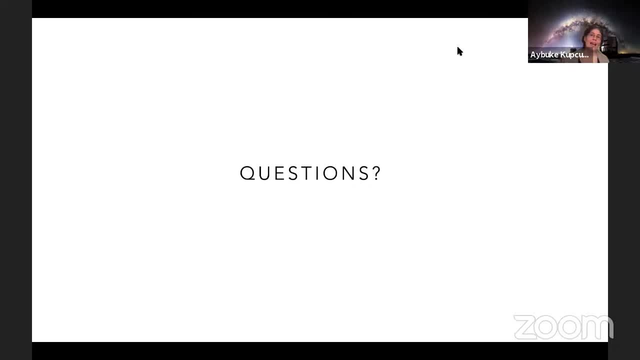 and you need to know, obviously, physics and astronomy, and then for theoretical astronomy, it's a different thing- you need to know more maths and more physics. so there are there are many different options and and different paths to um, yeah, yeah, wonderful i'm, i'm also going to, uh, shamelessly plug the.